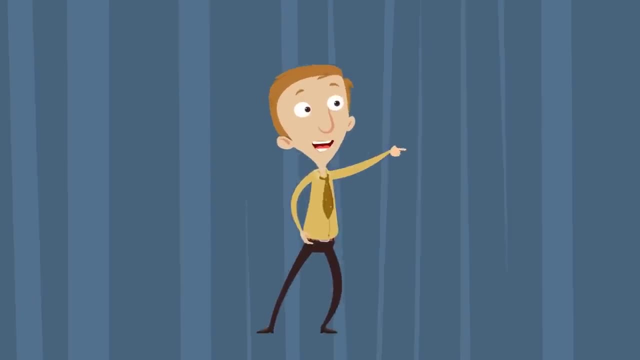 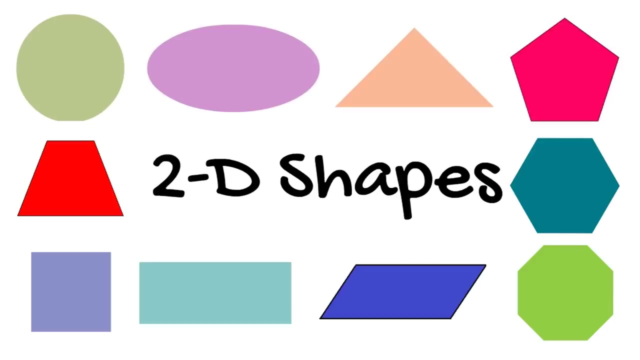 I really like this. You know I like to dance. You know some people they're not dancers. You know I dance, I dabble in dancing, you know. All right, that's enough. Can somebody turn that music off? I mean, seriously, I can't teach like this, I can't teach with this music going on. You 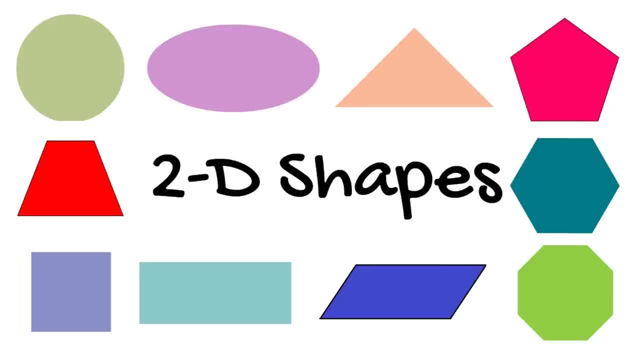 know I feel like I'm in a candy shop. Let's turn the music off, please, Thanks. So here they are, our old friends, the 2D shapes. You're familiar with these. you know You're familiar with the. 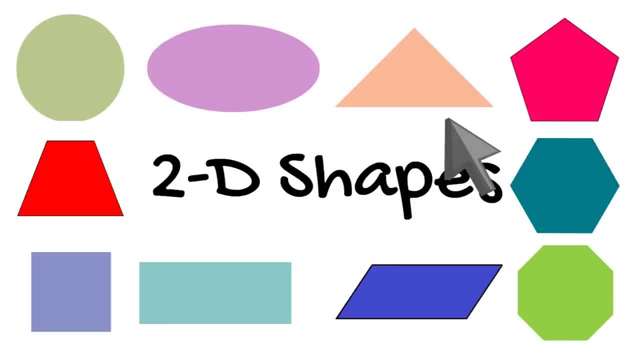 circle, the oval, the triangle, the pentagon, the trapezoid, the hexagon, the square, the rectangle, the parallelogram And the octagon. And these aren't all our shapes, our 2D shapes, you know, But these are all family. 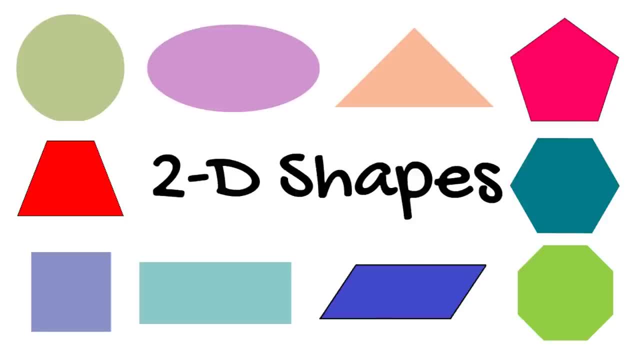 friends of ours. We don't want to just forget about these, And before we look at 3D shapes, it's really important for us to look at these shapes again, because these are old friends. So we're going to look at each one of these one by one, just to make sure you know who they are. 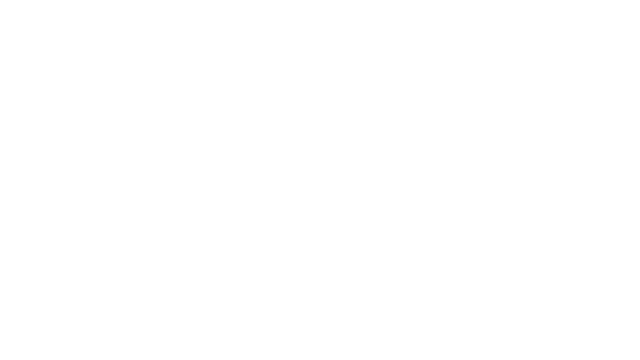 before we learn all these new shapes. This first shape doesn't even need an introduction. It's the circle. the circle, that round figure. It's awesome. We love this shape. It's one of the first ones we ever learn: The circle. This next shape is one of the stretchy shapes: the oval. 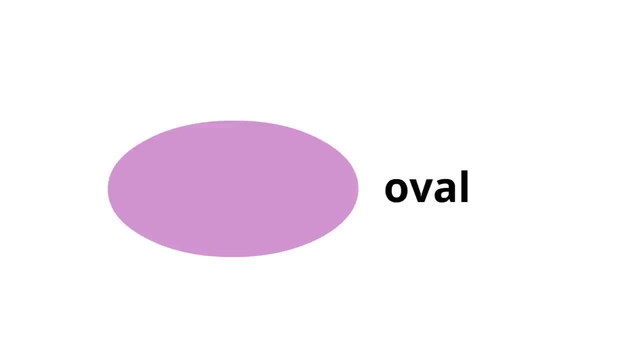 It's like a circle got stretched out. It's elongated, It's a tremendous shape, the oval. Here's another familiar shape: the triangle Triangle, Three sides. We love the triangle. The triangle is great. The three-sided friend Three. 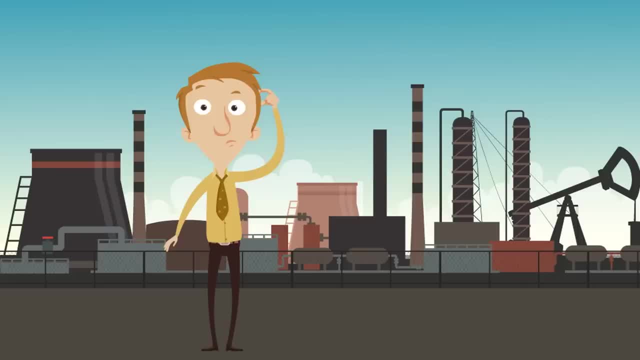 sides A triangle. Wait, I keep saying we love the shapes. I mean we like the shapes, but do you love the shapes? Do I love the shapes? I mean I don't know, I need to take it easy here. All right, 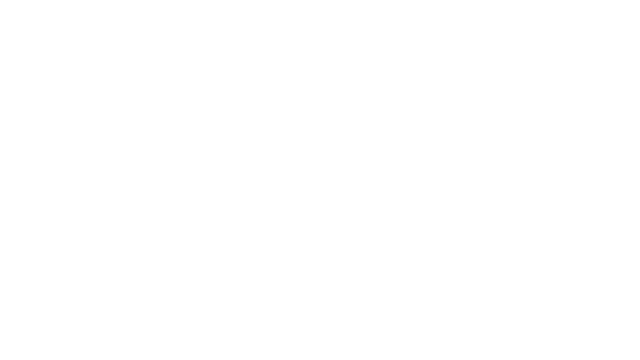 before we learn all these new shapes. This first shape doesn't even need an introduction. It's the circle. the circle, that round figure. It's awesome. We love this shape. It's one of the first ones we ever learn: The circle. This next shape is one of the stretchy shapes: the oval. 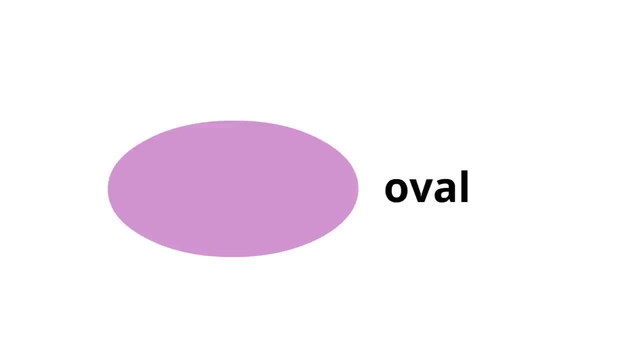 It's like a circle got stretched out. It's elongated, It's a tremendous shape, the oval. Here's another familiar shape: the triangle Triangle, Three sides. We love the triangle. The triangle is great. The three-sided friend Three. 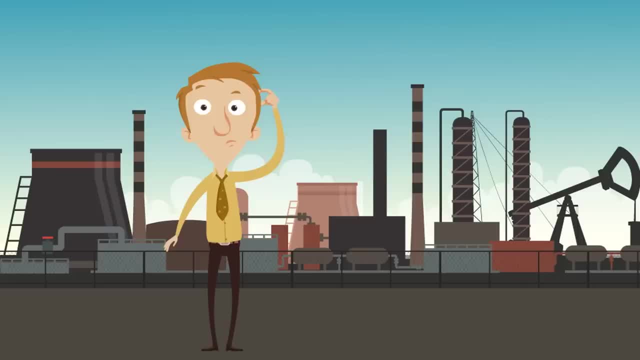 sides A triangle. Wait, I keep saying we love the shapes. I mean we like the shapes, but do you love the shapes? Do I love the shapes? I mean I don't know, I need to take it easy here. All right, 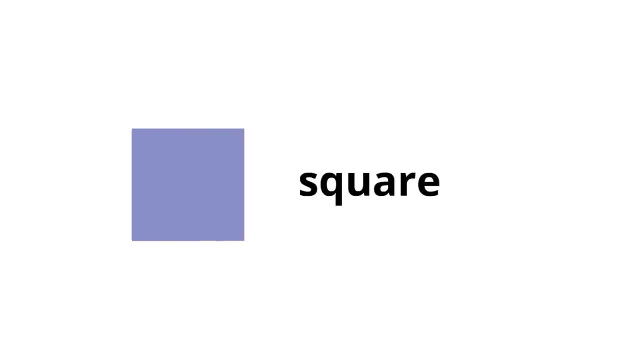 let's keep going. Ah, the square, Four sides all equal. You know, the square's good, The square's a good shape. you know, Sometimes you just need a square, Sometimes you just need a square. Here's the rectangle. The rectangle is longer than the square because not all four sides. 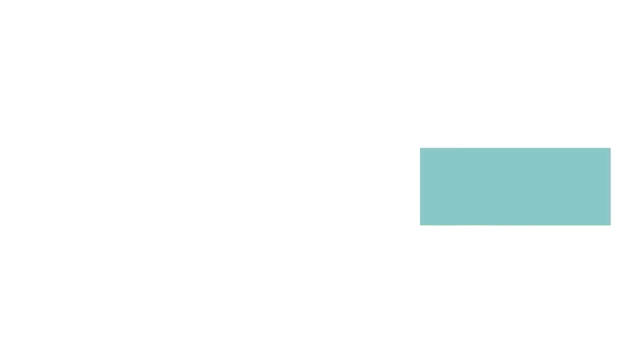 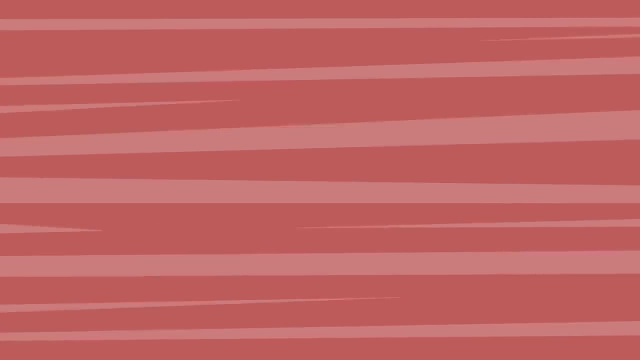 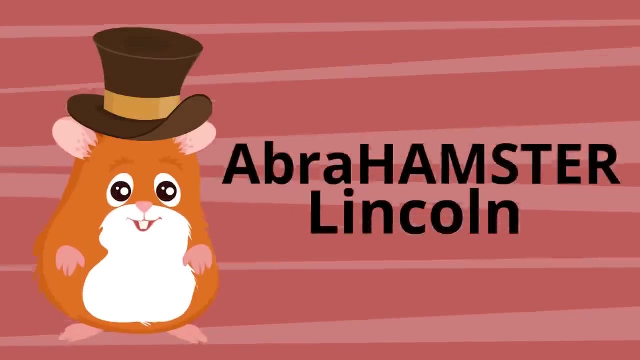 are equal: The rectangle. I know, I know, I know We're in the middle of something here, but I have to share this. Okay, So what do you call a hamster with a top hat? Abrahamster Lincoln? I digress. 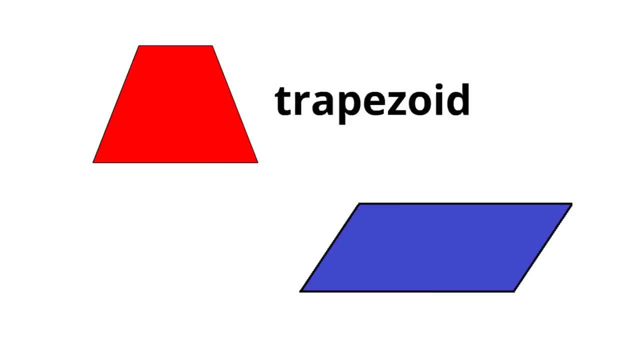 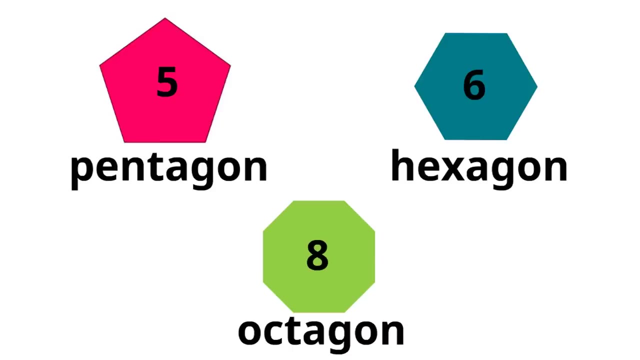 The trapezoid, a cool shape with two of the sides being parallel to each other. in the parallelogram, another four-sided shape, Both pairs of sides are parallel to each other. Okay, And finally the pentagon with five sides. 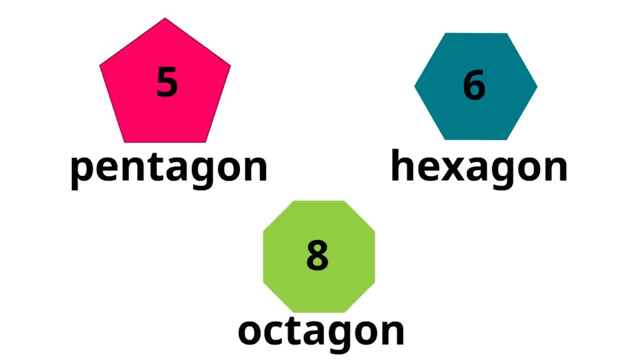 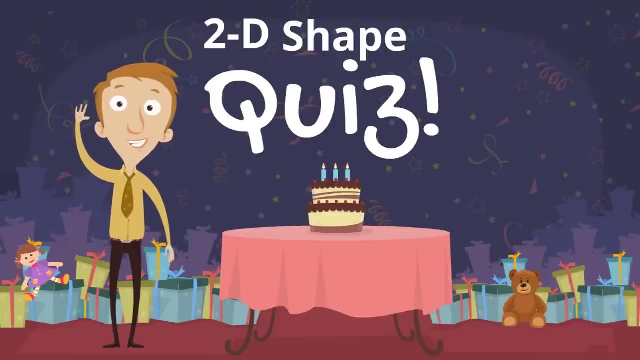 sides, the hexagon with six sides and the octagon with eight sides. what awesome shapes. so let's go ahead and do a quick 2d shape quiz. i need your help. i want to see if you really learned these, if you really know these, before we get into the 3d shape. so 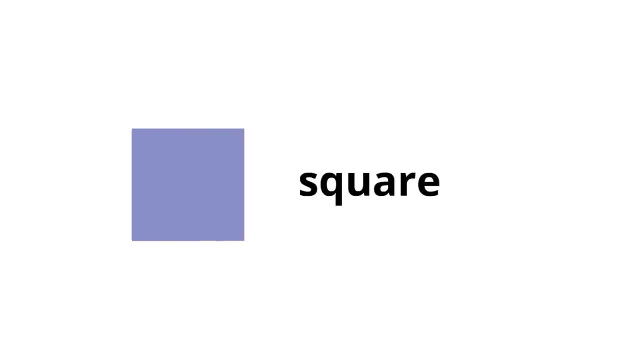 let's keep going. Ah, the square, Four sides all equal. You know, the square's good, The square's a good shape. you know, Sometimes you just need a square, Sometimes you just need a square. Here's the rectangle. The rectangle is longer than the square because not all four sides. 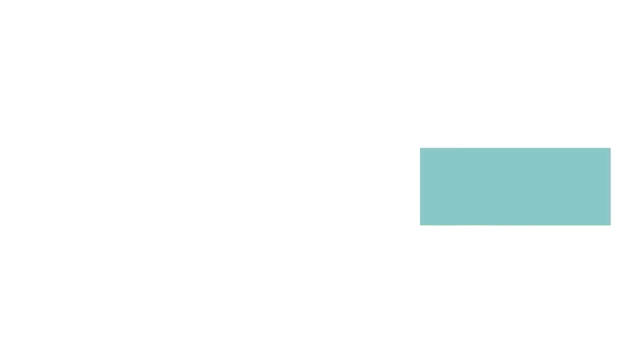 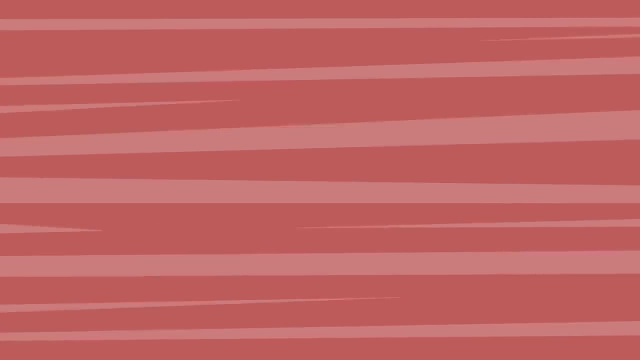 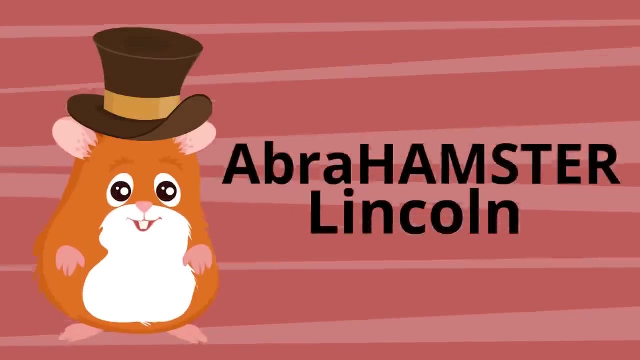 are equal: The rectangle. I know, I know, I know We're in the middle of something here, but I have to share this. Okay, So what do you call a hamster with a top hat? Abrahamster Lincoln? I digress. 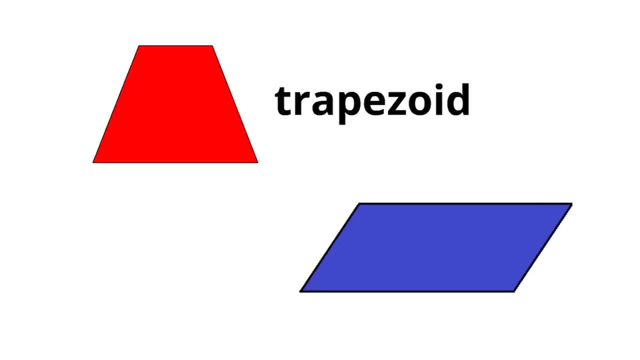 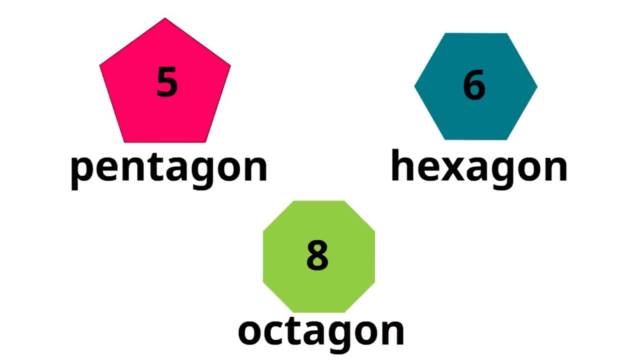 The trapezoid- a cool shape with two of the sides being parallel to each other. in the parallelogram, another four-sided shape, Both pairs of sides are parallel to each other. And finally the pentagon with five sides, the hexagon with six sides and the octagon with eight sides. What awesome shapes. 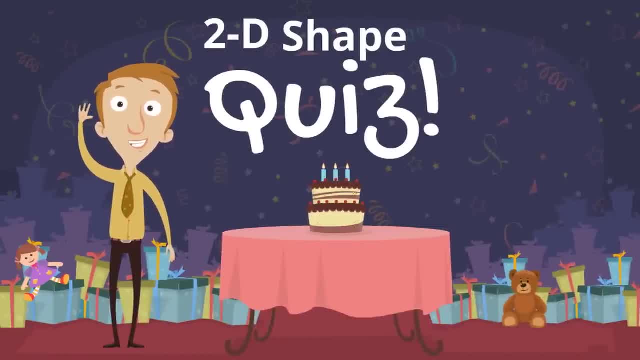 So let's go ahead and do a quick 2D shape quiz. I need your help. I want to see if you really learned these, if you really know these, before we get into the 3D shapes. So help me out here. 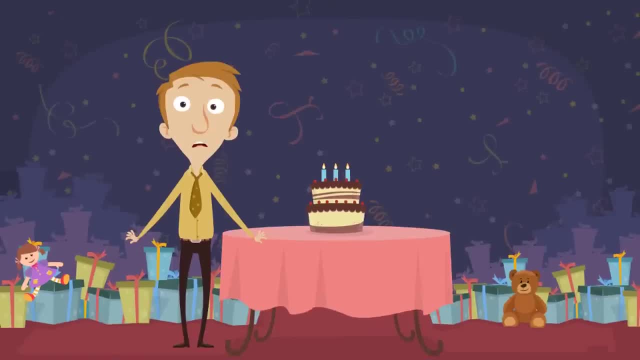 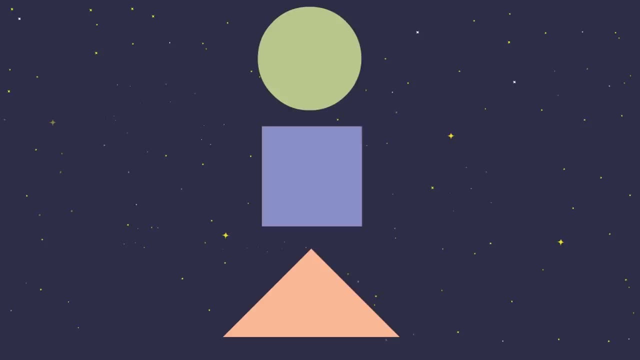 We're going to have an awesome time. Wait, what Is it my birthday, Oh well. What type of shape is on the top? Yeah, A circle. What type of shape is in the middle? Two A square, Awesome. Okay. now What shape is on the bottom? 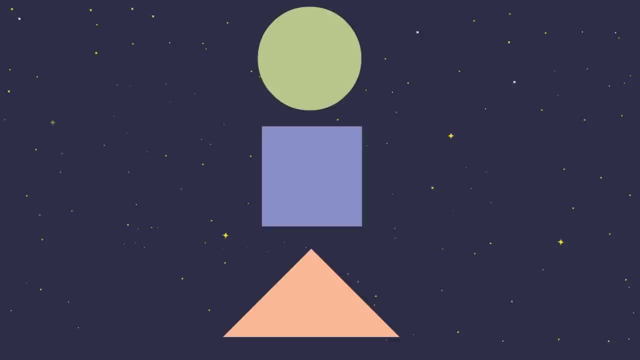 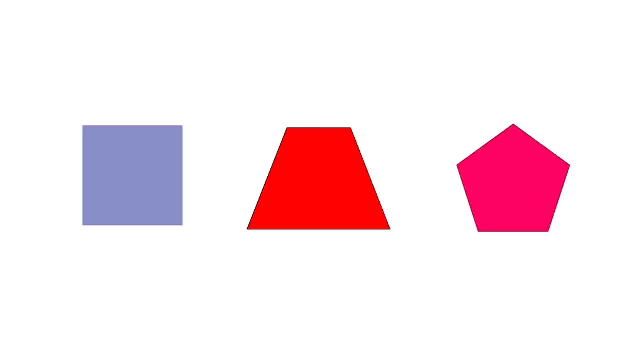 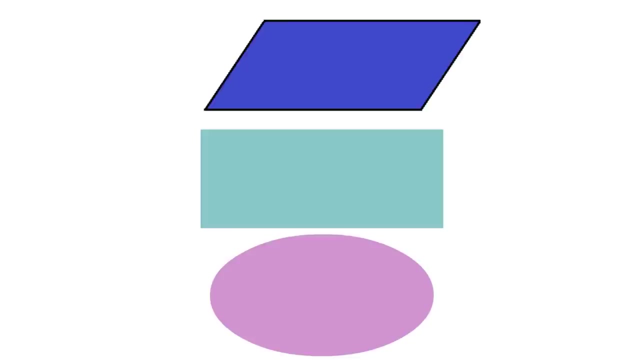 Three, Of course, A triangle, awesome job. now we've got more. this is a little trickier. which shape is in the middle? yeah, a trapezoid. which shape is on the right- the Pentagon- good job. and which shape is on the left? yeah, the square. now try these. which shape is on? 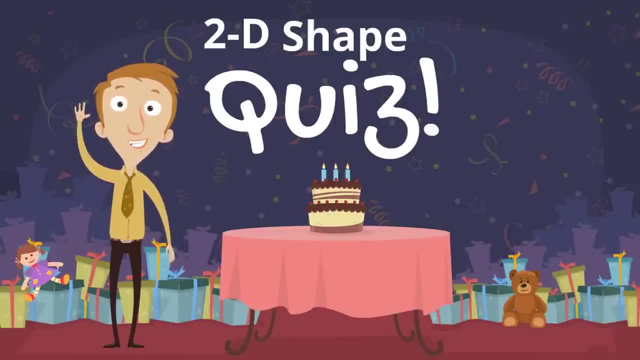 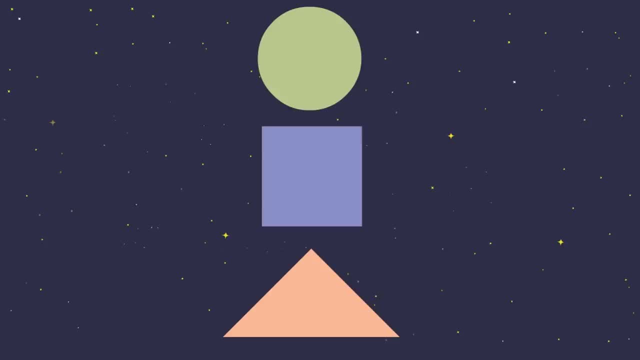 help me out here. we're gonna have an awesome time. wait what? it's not my birthday, oh well. what type of shape is on the top? yeah, a circle. what type of shape is in the middle? a square, awesome, okay. now what shape is on the bottom? of course, a triangle. awesome job, now we've got more. 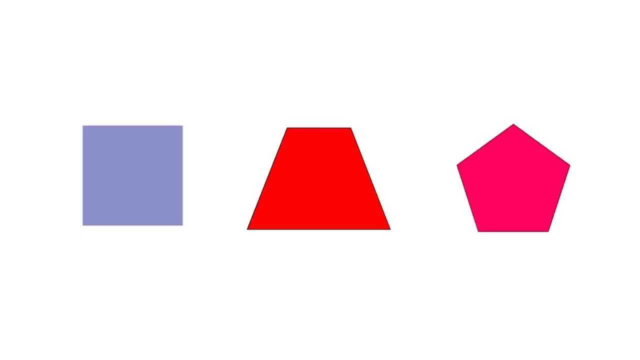 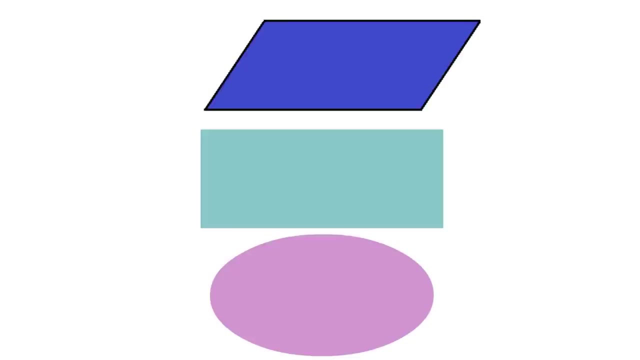 this is a little trickier. which shape is in the middle? yeah, a trapezoid. which shape is on the right- the pentagon- good job. and which shape is on the left? yeah, the square. now try these. which shape is on the bottom? yeah, the oval. which shape is on the top? 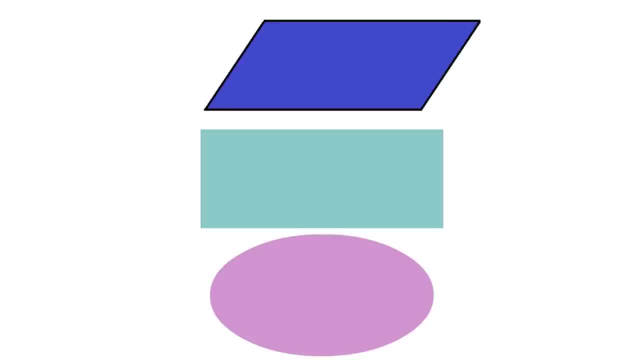 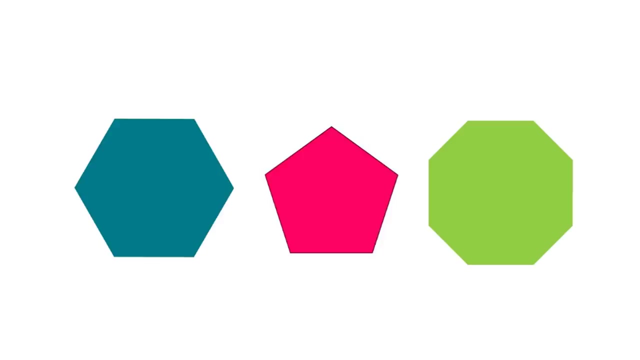 yeah, the parallelogram. which shape is in the middle is All right, the rectangle, great job, All right. the last one. Which shape is on the left? Yeah, the hexagon. Which shape is on the right? Great, the octagon. And which shape is in the middle? 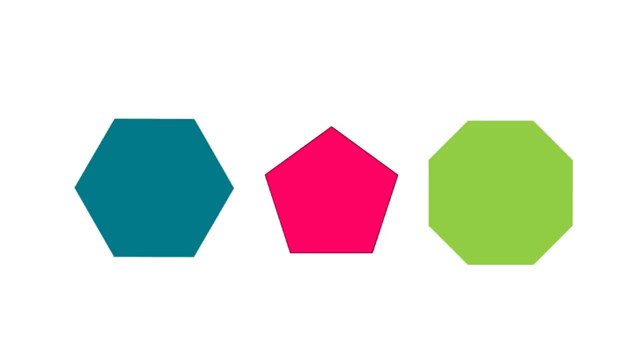 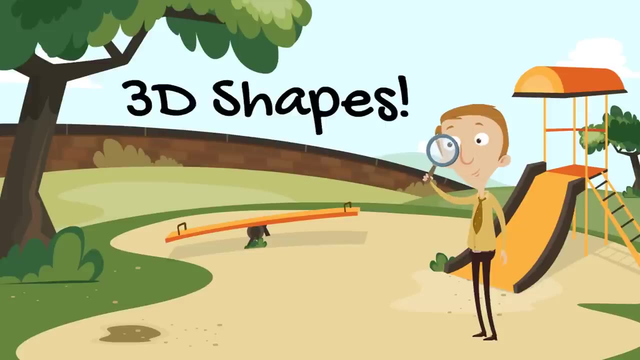 Phenomenal: the pentagon. All right, we're ready to learn the 3D shapes. We're going to learn how to identify the three-dimensional shapes. If you struggled through the quiz, you might want to watch the first part of the video again. 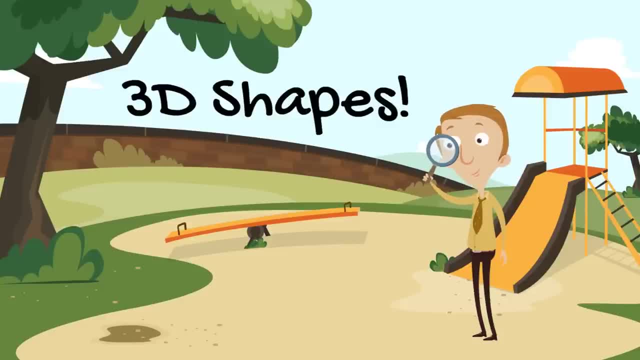 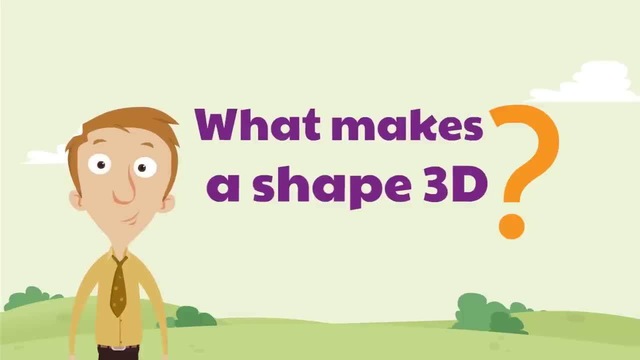 Otherwise, let's get started. So as we're starting out, it's important to remember What makes a 3D shape. What makes a 3D shape A 3D shape? There's an old rhyme that says 3D shapes are fat, not flat. 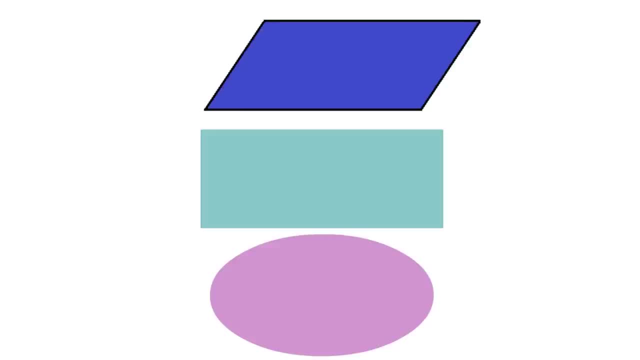 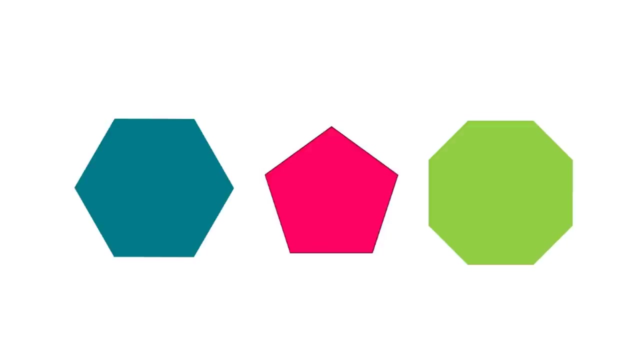 the bottom? yeah, the oval. which shape is on the top? yeah, the parallelogram. parallelogram. which shape is in the middle? all right, the rectangle, great job. all right, the last one. which shape is on the left? yeah, the hexagon. which shape is on the right? 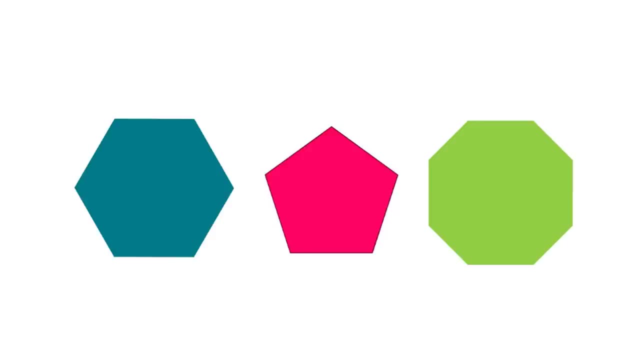 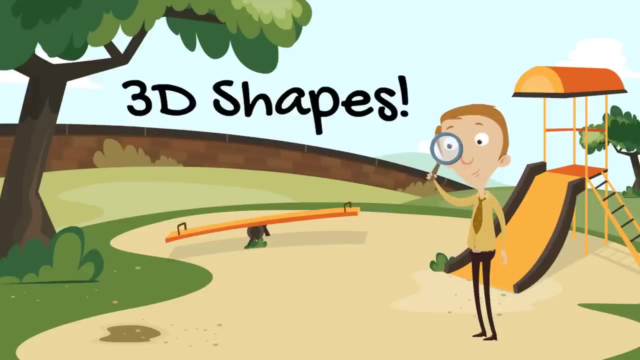 huay, the octagon, and which shape is in the middle? the nominal, the Pentagon? all right, we're ready to learn. the 3d ships were going to learn how to identify the three-dimensional shapes. if you struggle through the quiz, you might want to watch the first part of the video again. 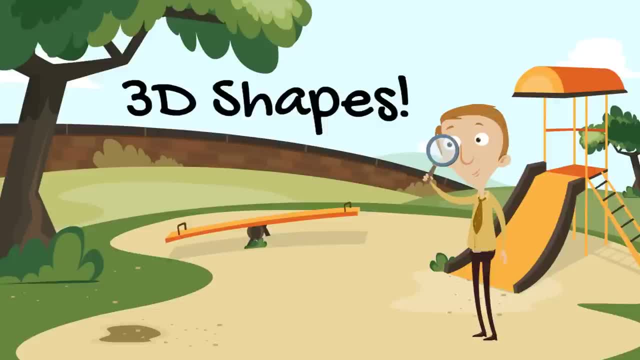 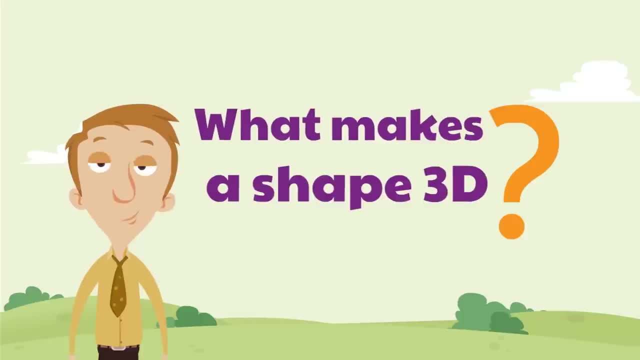 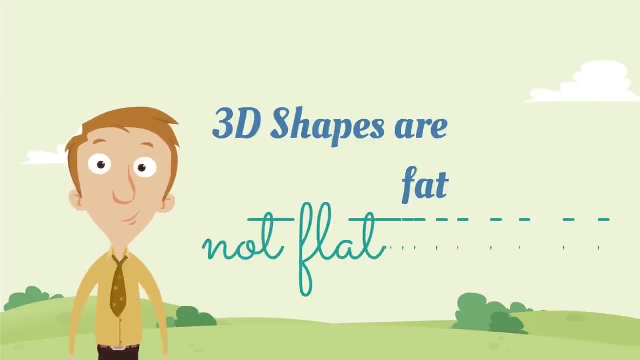 otherwise let's get started. so, as we're starting out, It's important to remember what makes a 3D shape a 3D shape. There's an old rhyme that says 3D shapes are fat, not flat, And you can see that with the sphere, which is a 3D shape, we're about to learn, and the circle. 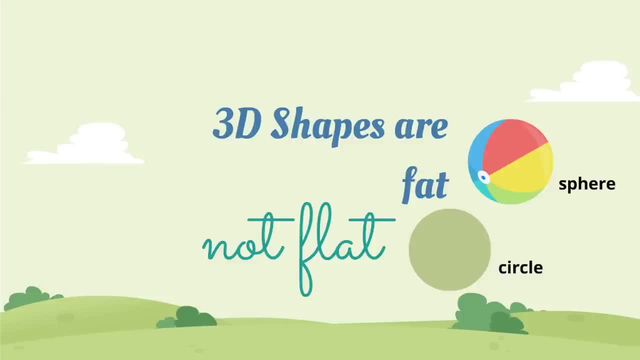 The circle is flat, but the sphere is 3D, It's three-dimensional. All the shapes are like that, So let's learn all these 3D shapes. So the first 3D shape we're going to learn is the sphere, the one that we just mentioned. 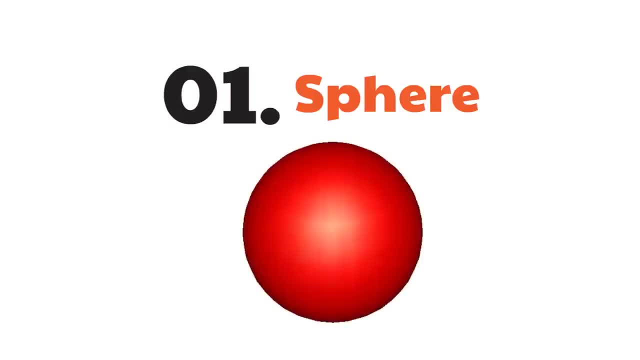 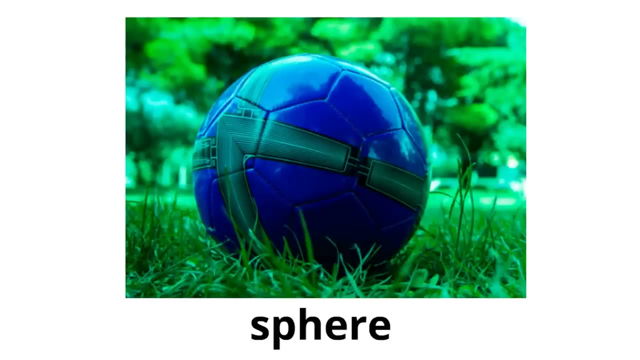 The sphere is the 3D version of the circle. It's perfectly round. There are spheres all around us. One of the spheres we see all the time are balls like this soccer ball. A soccer ball is a sphere. It's perfectly round. 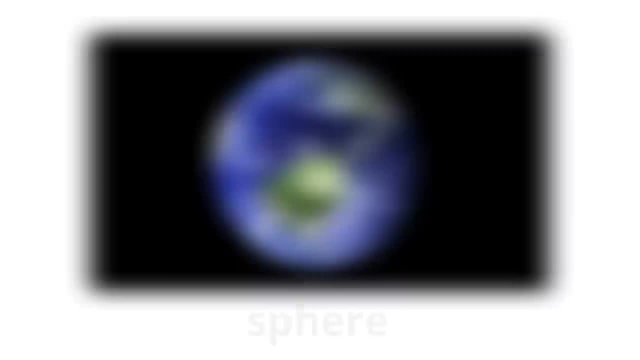 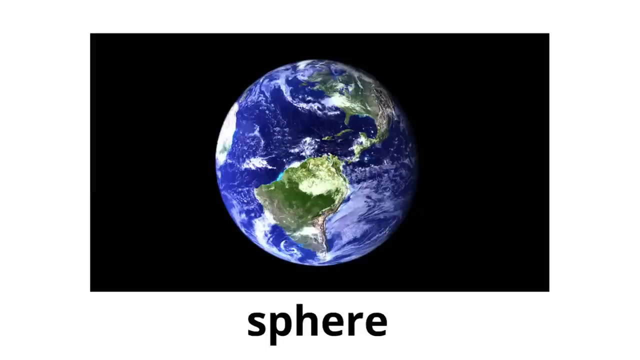 It's a 3D circle, It's a sphere. You know this sphere? Yes, it's the Earth. It's where we live. Our planet is a sphere. How cool is that? Our own planet is a sphere, Perfectly round. 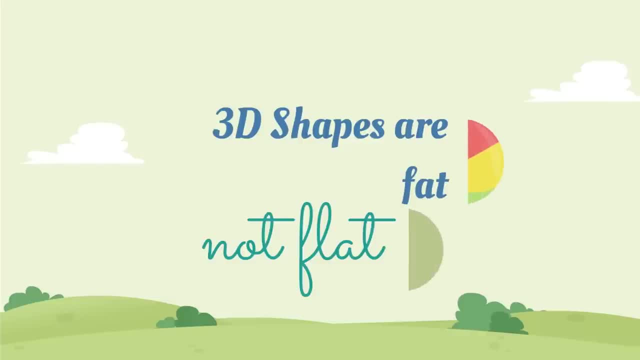 And you can see that with the sphere, Which is a 3D shape we're about to learn, And the circle. The circle is flat, But the sphere is 3D, It's three-dimensional. All the shapes are like that. So let's learn all these 3D shapes. 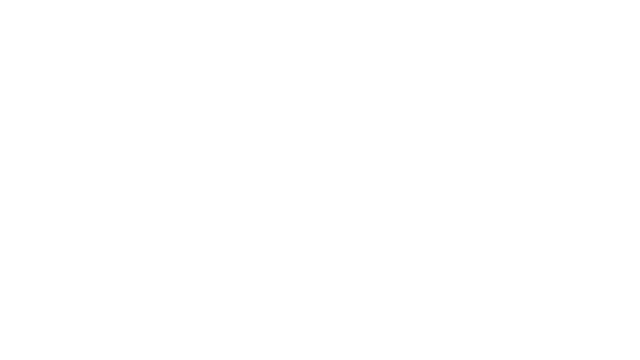 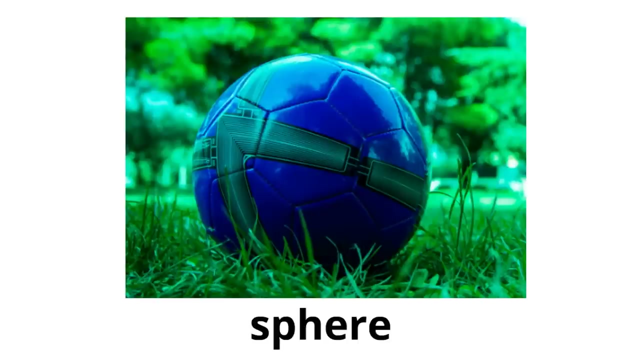 So the first 3D shape we're going to learn Is the sphere, The one that we just mentioned. The sphere is the 3D version of the circle. It's perfectly round. There are spheres all around us. One of the spheres we see all the time. 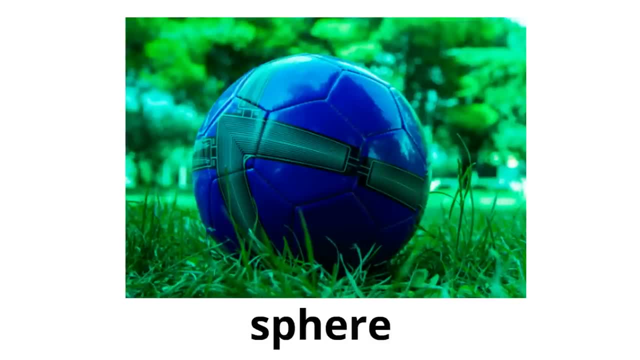 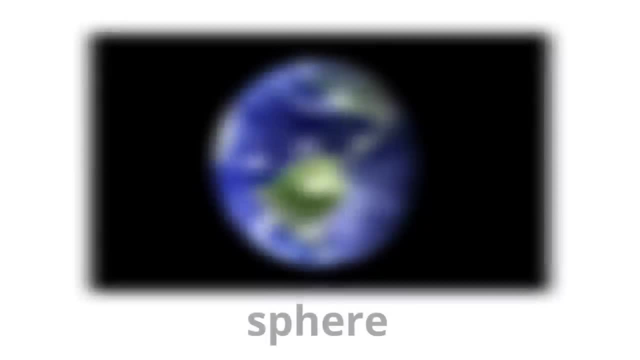 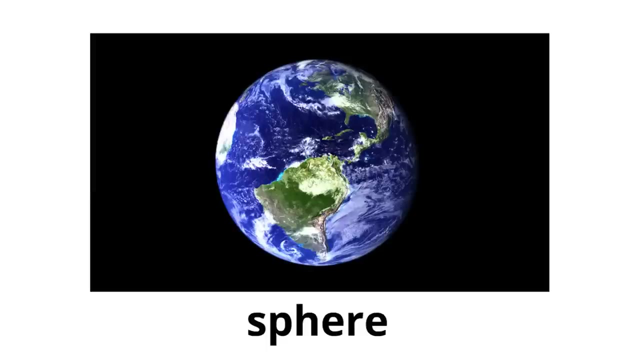 Are balls like this soccer ball. A soccer ball is a sphere. It's perfectly round. It's a 3D circle. It's a sphere. You know this sphere? Yes, it's the earth. It's where we live. Our planet is a sphere. How cool is that. 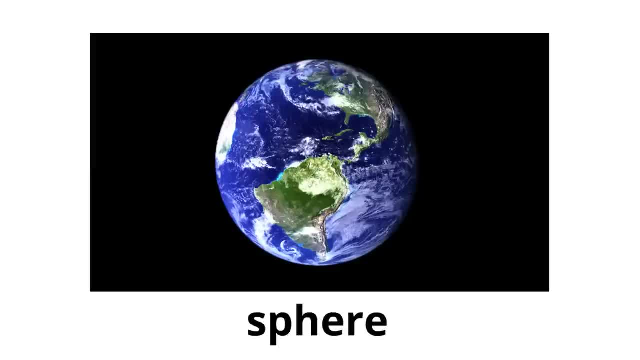 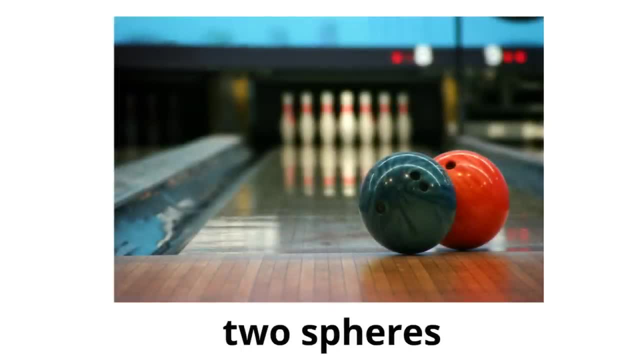 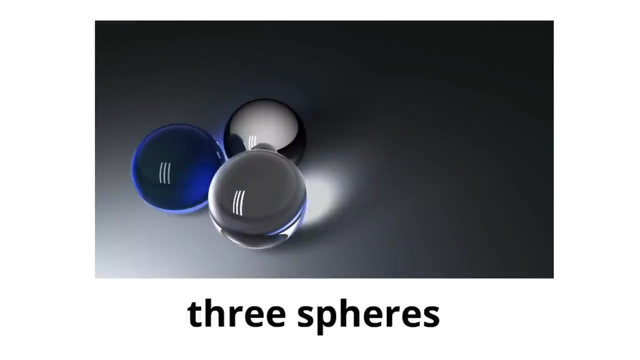 Our own planet is a sphere, Perfectly round. It's a sphere. In this picture we have two spheres. Can you spot them? Yeah, The two spheres are the two bowling balls- Perfect round spheres. Spheres are all around us. Here we have a group of three spheres. 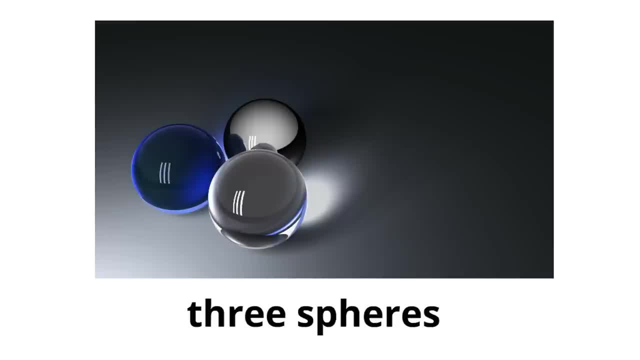 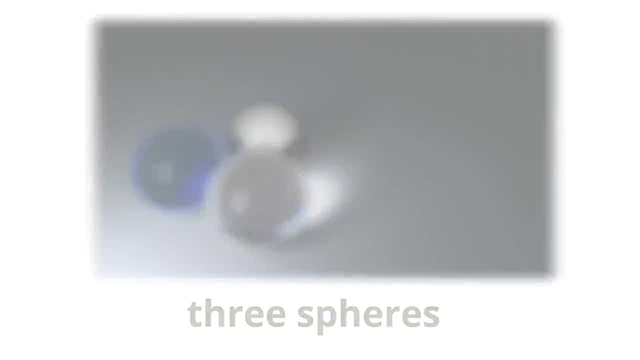 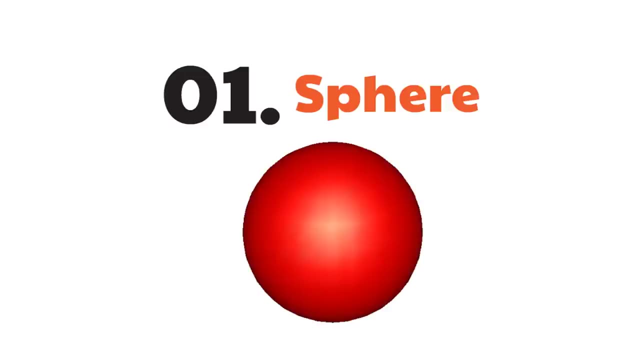 Spheres. You can count them right now: One, two, three spheres. all together The shape of a ball, A sphere, Perfectly round. Well, there you have it, The sphere. What a cool 3D shape. to start with, It's round. There are examples all around us. 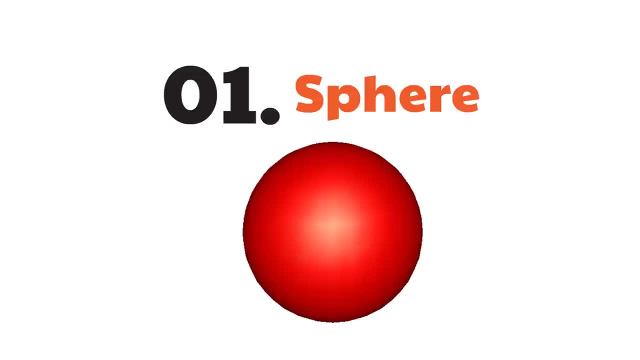 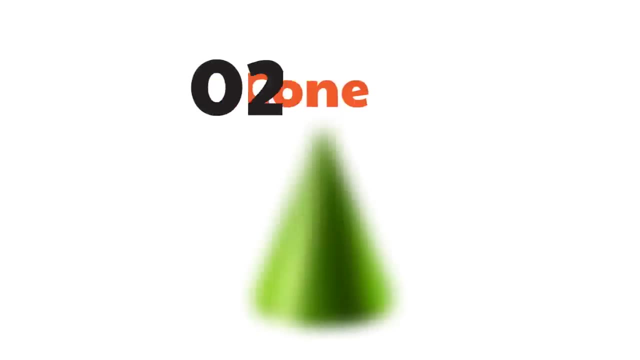 And it's just so cool And you know what The 3D shapes are going to get even better. Our second 3D shape is the cone. The cone is a really cool shape With a circle as the base or the bottom, And it all comes up to one point called a vertex. 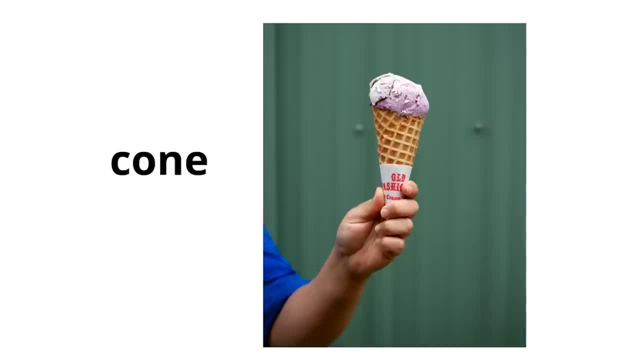 Here's an example of a cone. I think we all love The ice cream cone. If it doesn't have any ice cream inside And you flipped it upside down, You'd be able to see the circle base And it all comes up to one point called the vertex. 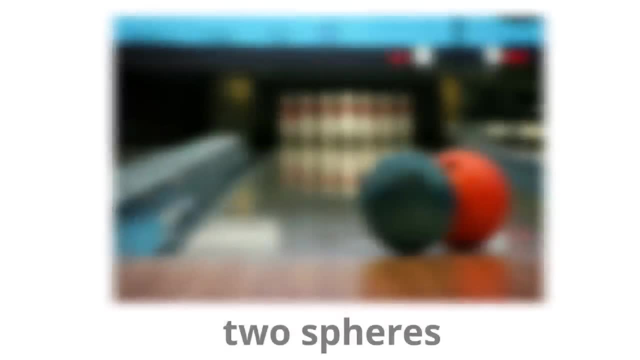 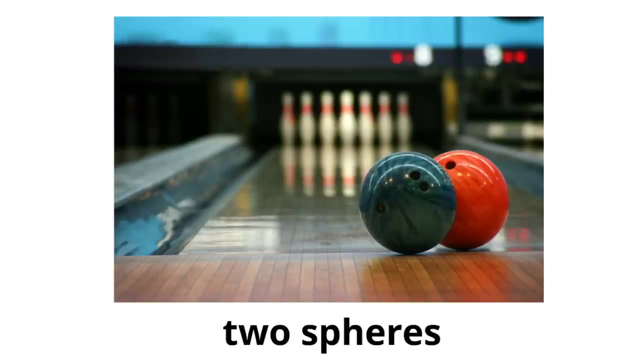 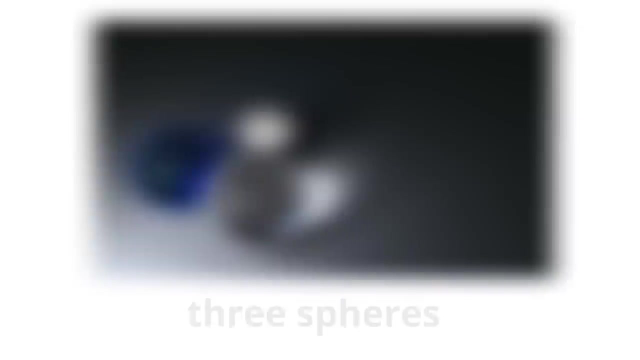 It's a sphere In this picture. we have two spheres. Can you spot them? Yeah, The two spheres are the two bowling balls. Perfect, round spheres. Spheres are all around us Here. we have a group of three spheres. You can count them right now. 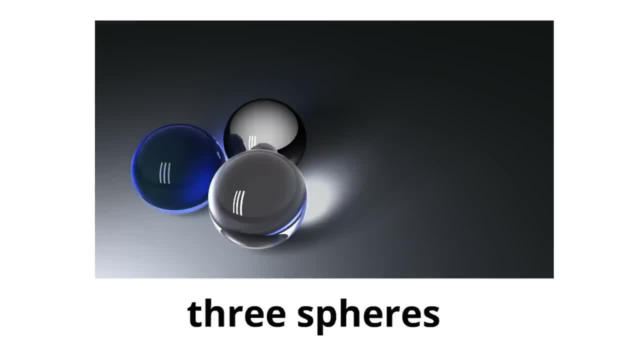 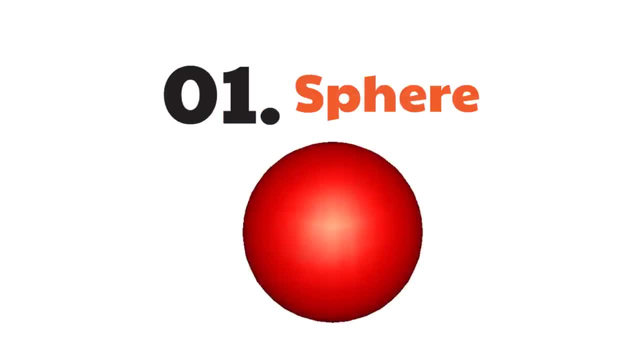 One, two, three spheres all together, The shape of a ball, a sphere, Perfectly round. Well, there you have it, The sphere. What a cool 3D shape. to start with, It's round. There are examples all around us. 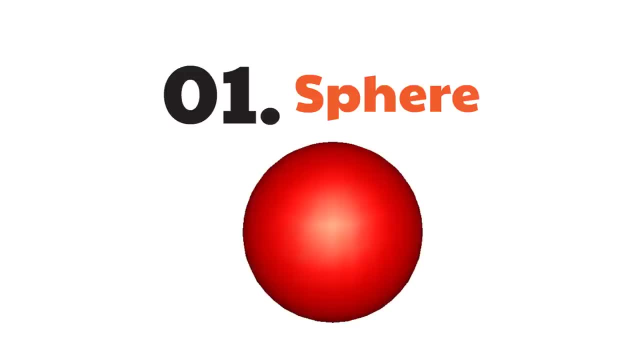 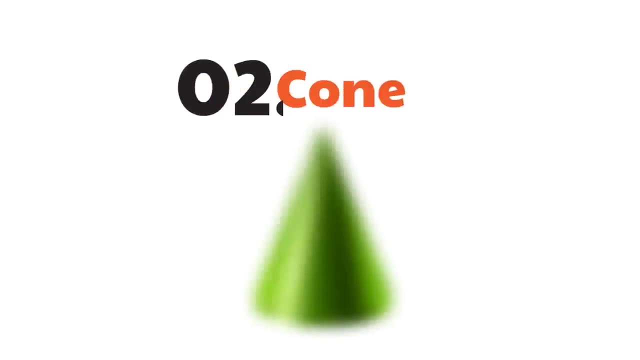 It's just so cool. You know what The 3D shapes are going to get even better. Our second 3D shape is the cone. The cone is a really cool shape with a circle as the base or the bottom, and it all comes. 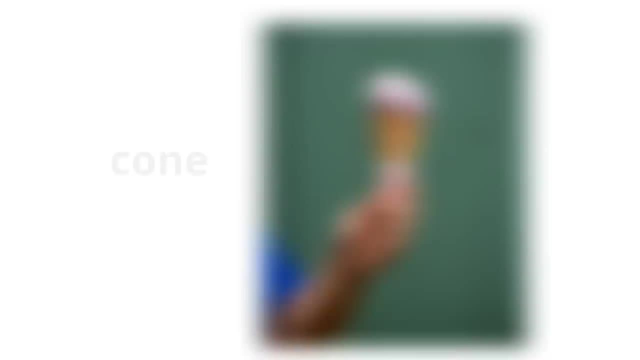 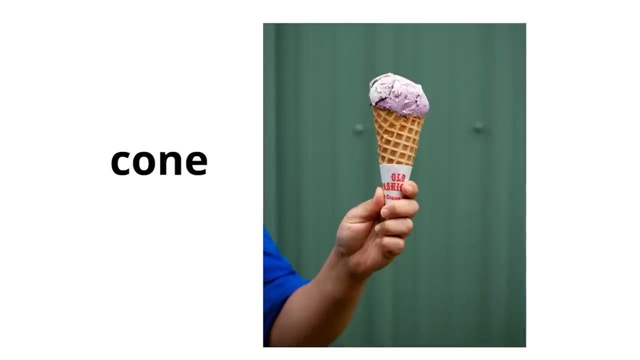 up to one point called a vertex. Here's an example of a cone. I think we all love The ice cream cone If it doesn't have any ice cream inside and you flipped it upside down, you'd be able to see the circle base and it all comes up to one point called the vertex. 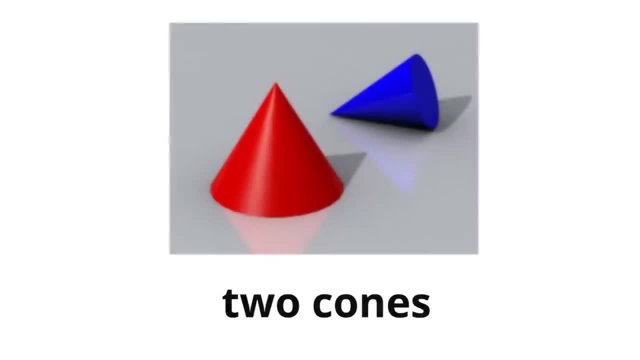 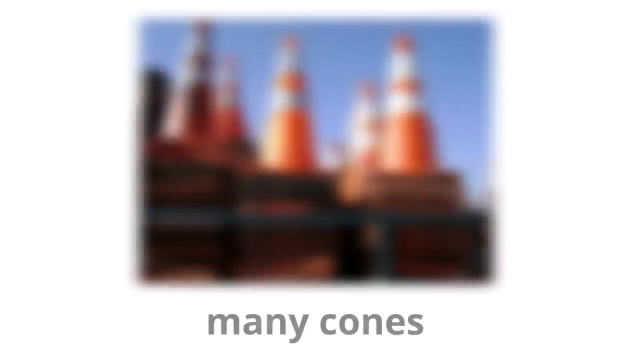 Perfect. Here are two cones, a red cone and a blue cone, and you can see both cones have that circle base and it all comes up to a vertex. What wonderful cones. Have you seen these before? They're traffic cones. Here are many cones. 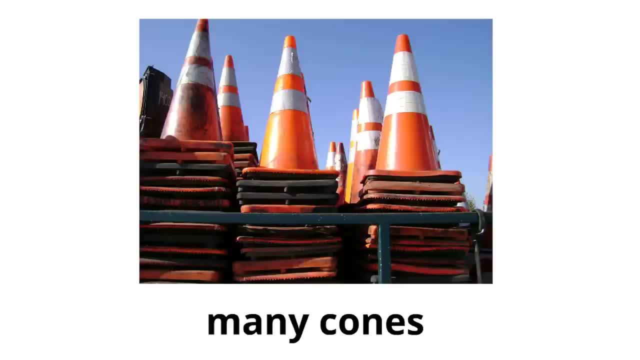 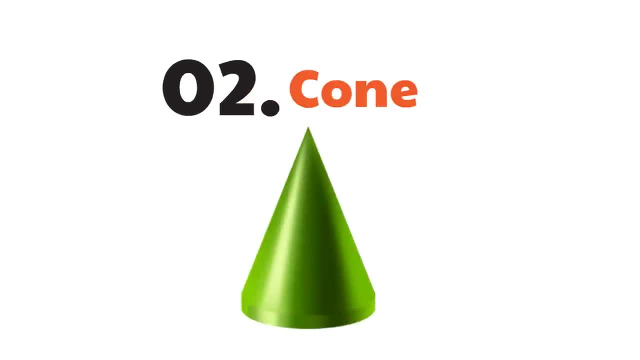 I didn't count all of them, but there's a lot and they're wonderful, wonderful cones. So that's our second 3D shape: the cone, a wonderful cone with a great circle base. It all comes up to one point called the vertex. 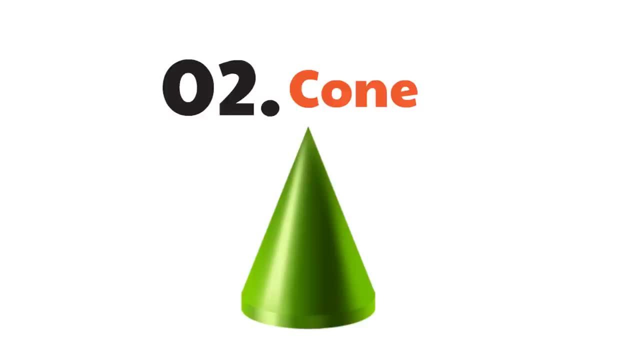 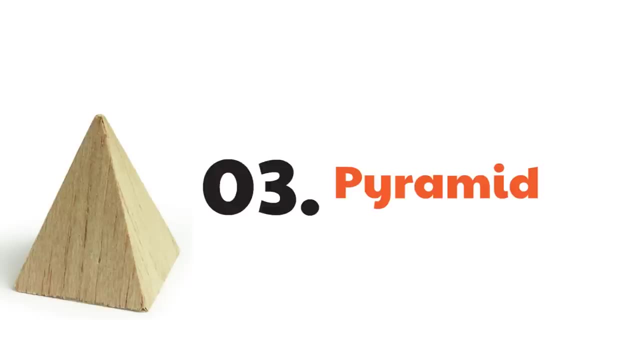 How awesome is that? Our third 3D shape is the pyramid. I love the pyramid. The pyramid's great. It comes up to one point, just like the cone, except the base is a square and the sides, instead of being smooth, they are triangles. 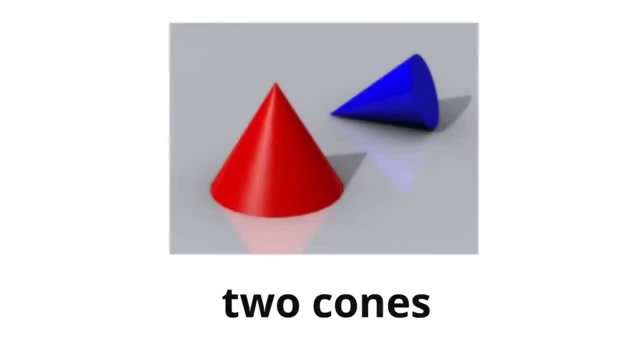 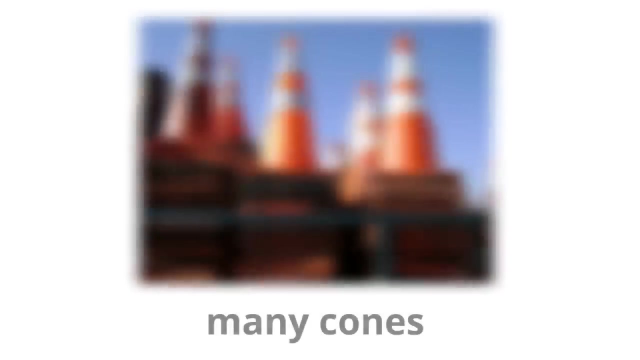 Here are two cones, A red cone And a blue cone, And you can see both cones have that circle base And it all comes up to a vertex. What wonderful cones. Have you seen these before? They're traffic cones. Here are many cones. I didn't count all of them. 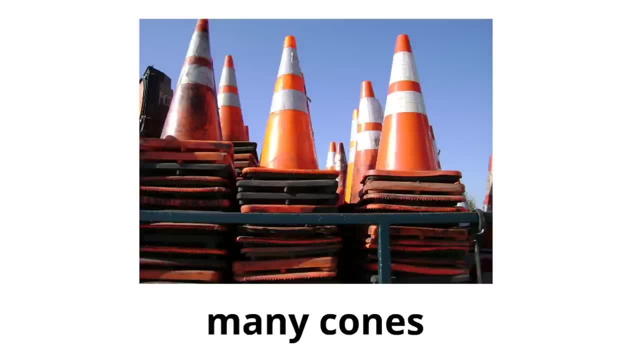 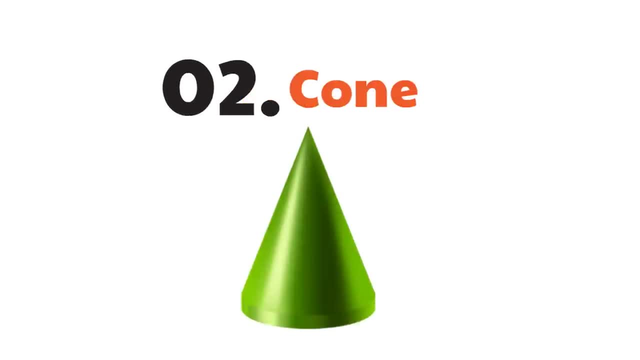 But there's a lot And they're wonderful, wonderful cones. So that's our second 3D shape, The cone. It's a wonderful cone With a great circle base. It all comes up to one point called the vertex. How awesome is that? Our third 3D shape is the pyramid. 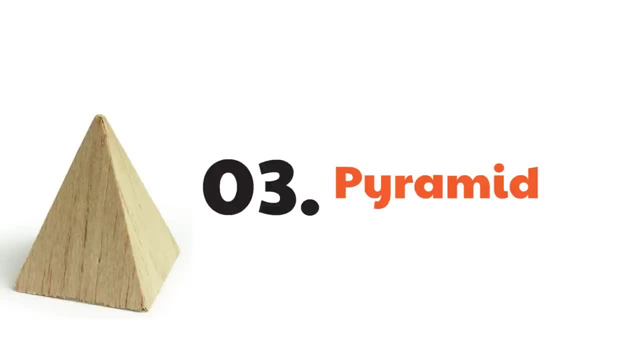 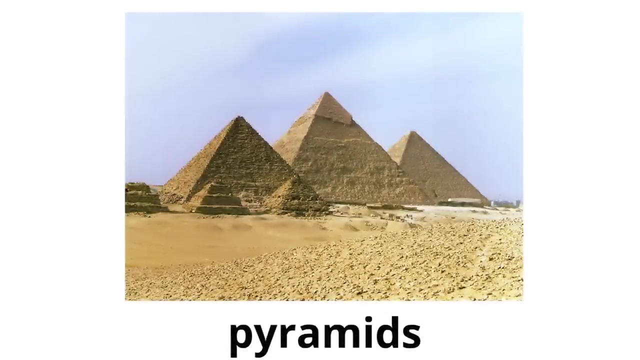 I love the pyramid. The pyramid's great. It comes up to one point, Just like the cone, Except the base is a square And the sides, instead of being smooth, They are triangles. Okay, like these are awesome, These are so cool. The pyramids of Egypt. You see that they have the triangle sides. 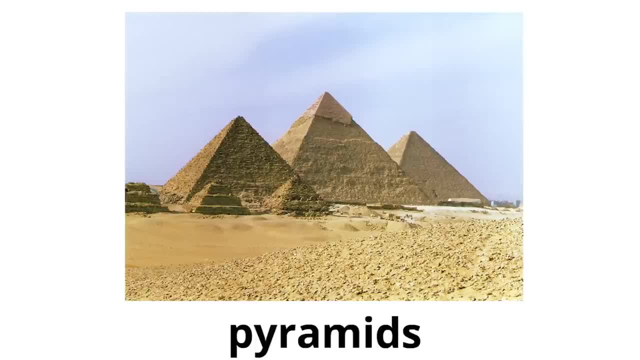 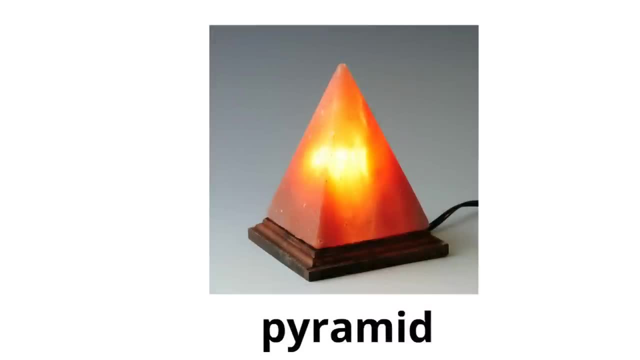 And the bottoms of these pyramids are square. They're awesome examples of the pyramid. This is a pretty cool pyramid. It's a decoration that you plug into the wall, But it's a great example of what a pyramid looks like. The bottom, or the base, is square. 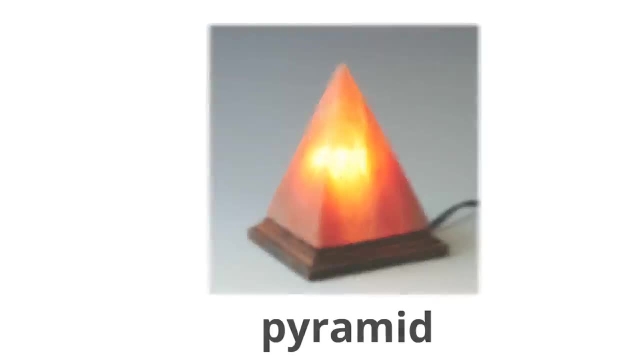 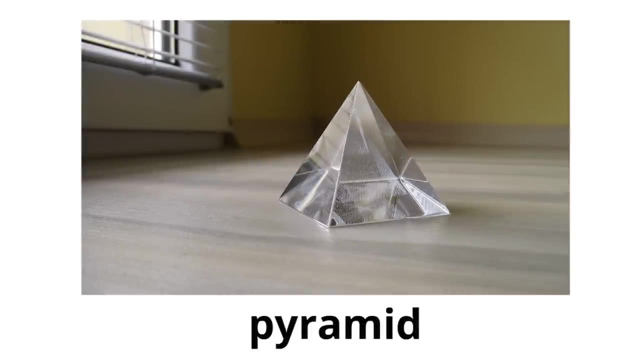 And there's the triangles on the sides. How cool is this? Here's another pyramid, And it's made of glass. There are so many decorations and things around, Maybe even your house, that are shaped like a pyramid. Because pyramids look so cool, People love putting them everywhere. 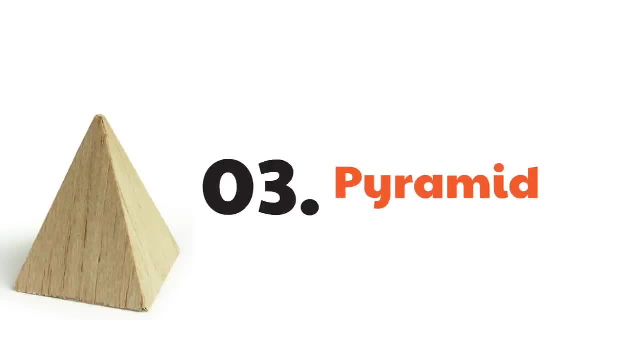 And there you go. I mean, you know the pyramid, It's a good shape. You know, you see a lot of them around. They've got the square bottom or base And the triangles on the sides And it all goes up to a vertex. It's a classic shape. 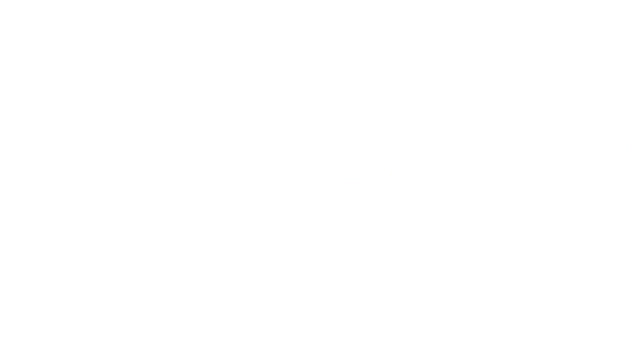 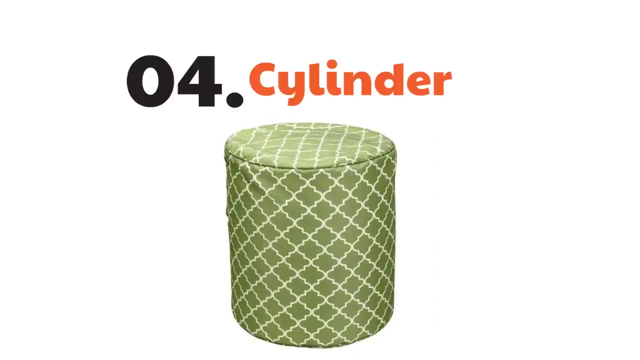 It's pretty awesome. Our fourth 3D shape is this: It's a cylinder. Now, a cylinder is easy to spot Because it's got a circle on the top And a circle on the bottom And it's smooth all around. Here we have a can of soup. 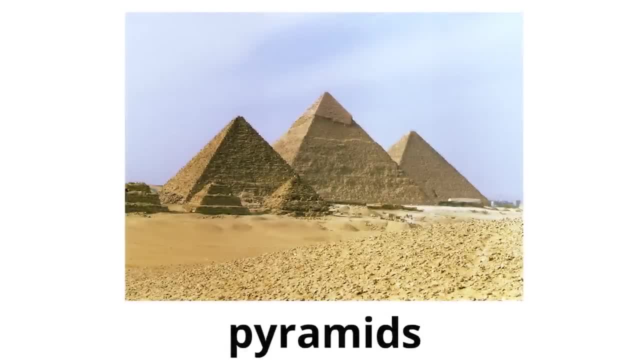 Okay, like these are awesome. These are so cool. The pyramids of Egypt. you see that they have the triangle sides and the bottoms of these pyramids are square. They're awesome examples of the pyramid. This is a pretty cool pyramid. 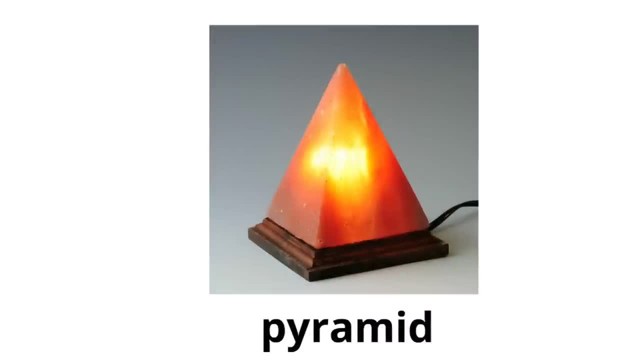 It's a decoration that you plug into the wall, but it's a great example of what a pyramid looks like. The bottom, or the base, is square and there's the triangles on the sides. How cool is this? Here's another pyramid, and it's made of glass. 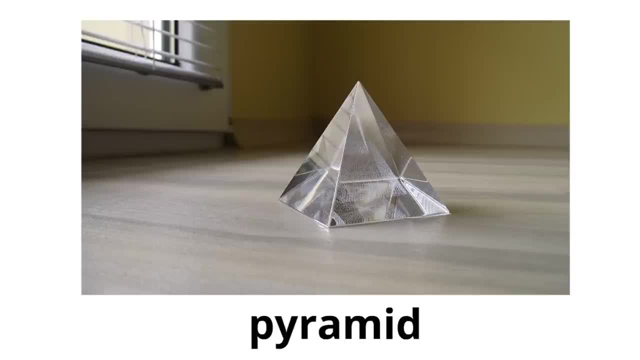 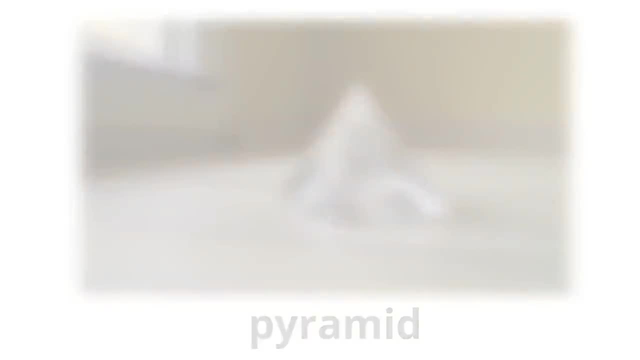 There are so many decorations and things around, maybe even your house, that are shaped like a pyramid. because pyramids look so cool, People love putting them everywhere. There you go. I mean, you know the pyramid, it's a good shape, You know you see a lot of them around. 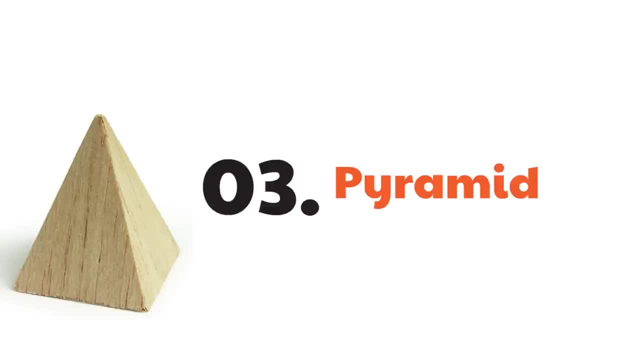 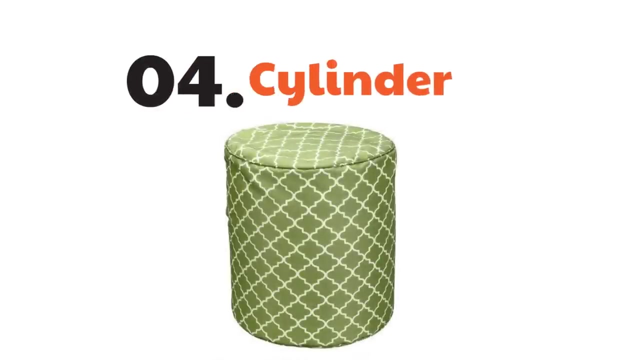 They've got the square bottom or base and the triangles on the sides and it all goes up to a vertex. It's a classic shape. It's pretty awesome. Our fourth 3D shape is the cylinder. Now, a cylinder is easy to spot because it's got a circle on the top and a circle on the. 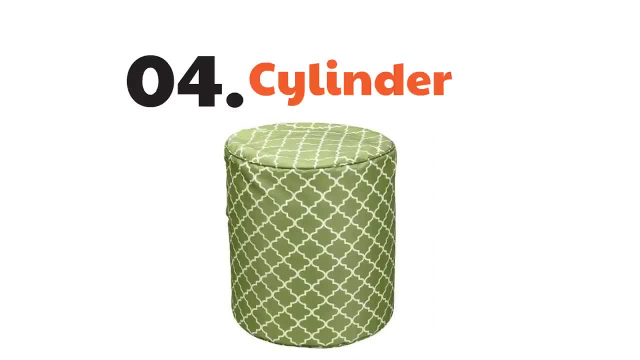 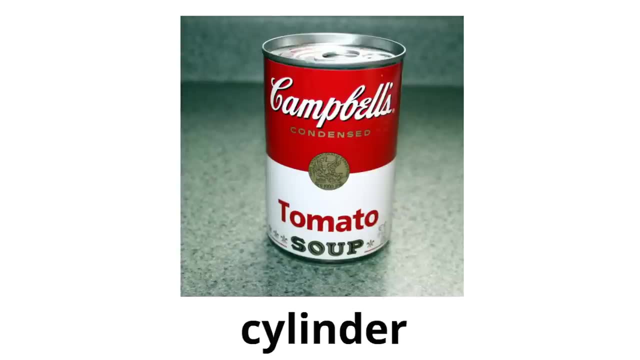 bottom and it's smooth all around. Here we have a can of soup and it's a cylinder. It has a circle on the top, a circle on the bottom and it's smooth all around. All cans and most jars are cylinders- Three cylinders. 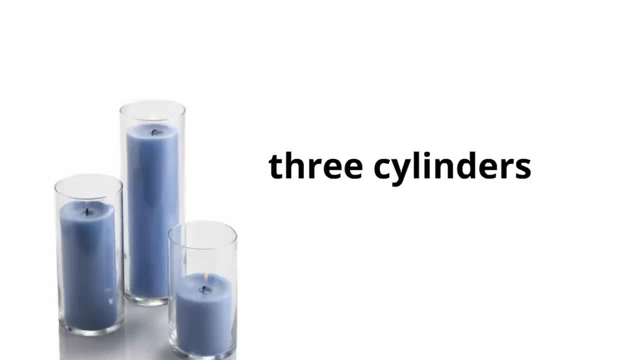 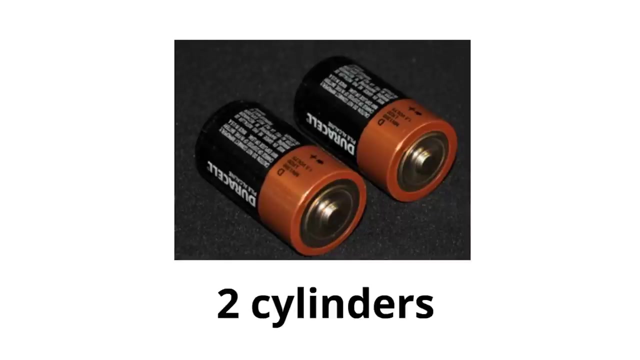 They're candles. And can I tell you a secret, Most candles are cylinders, too right? Oh, my goodness, this is just too crazy and too awesome. Here are two more cylinders. Are you kidding me? Are you kidding me? Even batteries are cylinders. 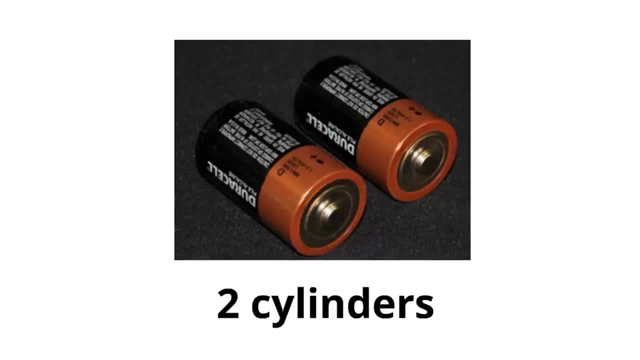 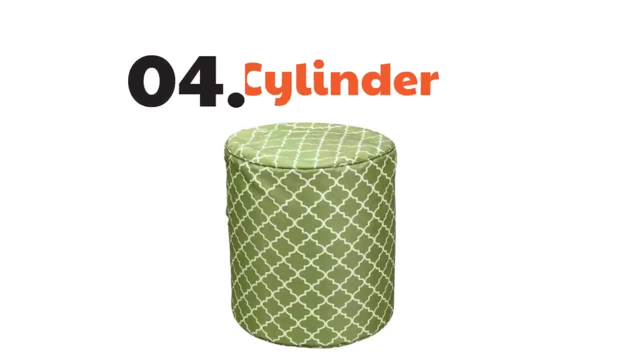 Cylinders are seriously everywhere: A circle on the top, a circle on the bottom and smooth all around. I mean really The cylinder is everywhere. I mean, you know, the circle on the top, circle on the bottom, smooth, all around. 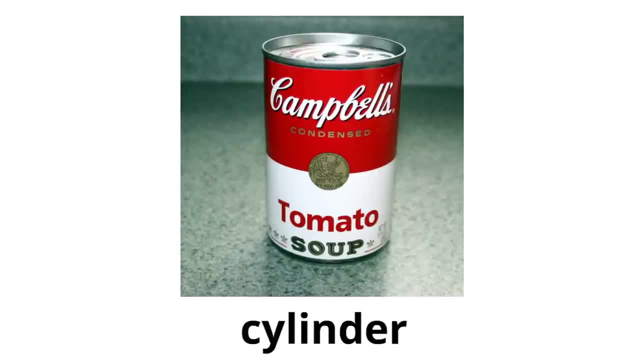 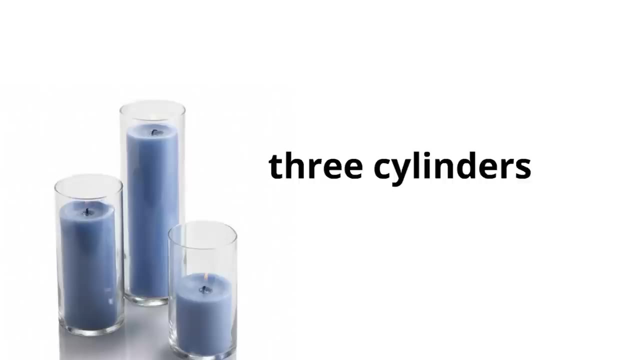 And it's a cylinder. It has a circle on the top, A circle on the bottom And it's smooth all around. All cans and most jars are cylinders. Here we have three cylinders. They're candles And can I tell you a secret, Most candles are cylinders too, right? 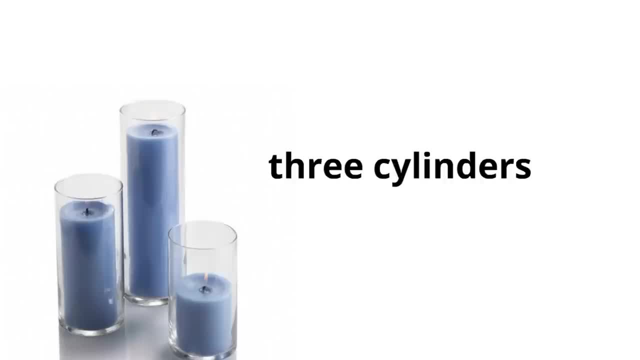 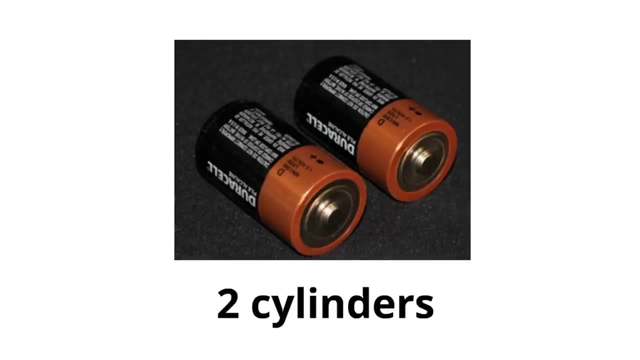 Oh, my goodness, This is just too crazy and too awesome. Here are two more cylinders. Are you kidding me? Are you kidding me? Even batteries are cylinders. Cylinders are seriously everywhere: A circle on the top, A circle on the bottom, And smooth all around. 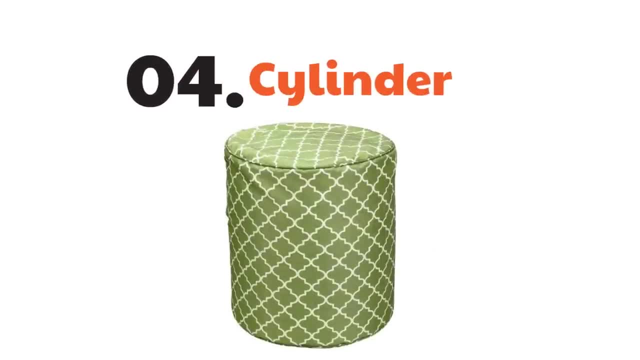 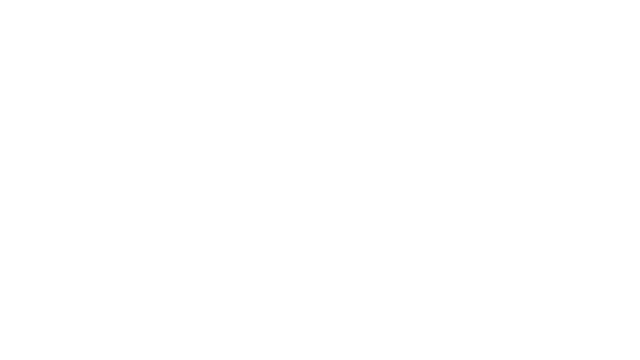 I mean, really, The cylinder is everywhere. I mean, you know, The circle on the top, Circle on the bottom, Smooth all around I I Cylinder. Like what in the world Do you have to be everywhere? okay, The next 3D shape is the cube. 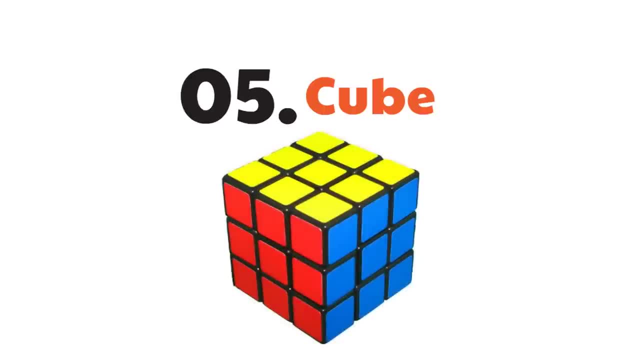 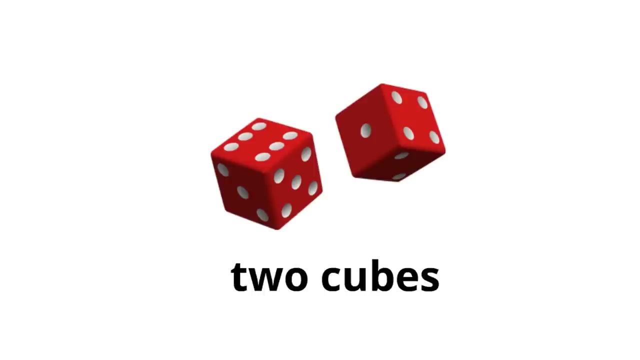 The cube is the 3D version of the square. It has six sides or faces That are all squares. Here we have two dice. Dice, Dice are in the shape of a cube. So these two dice are two cubes. They have six sides or faces That are all squares. 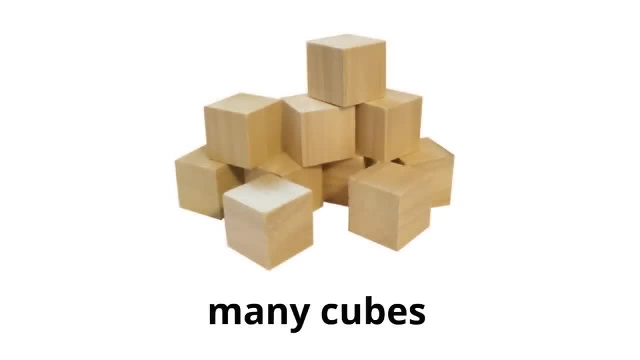 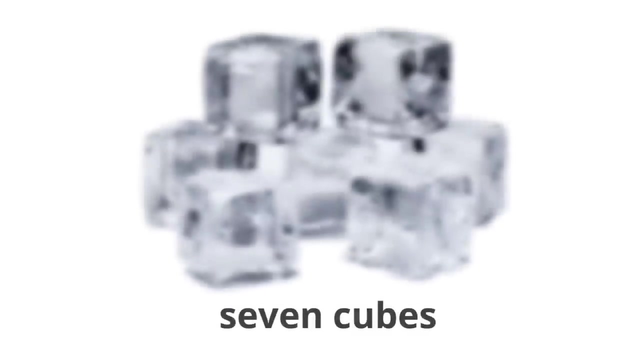 Here we have many cubes. These are cubes that are made out of wood. Each of them have six sides or faces That are all squares. Here are seven cubes of ice Ice. You ever had a warm drink and you need to put ice in it. It's awesome because it has this great shape. 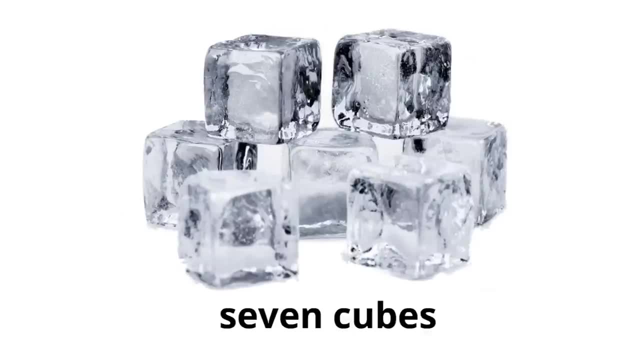 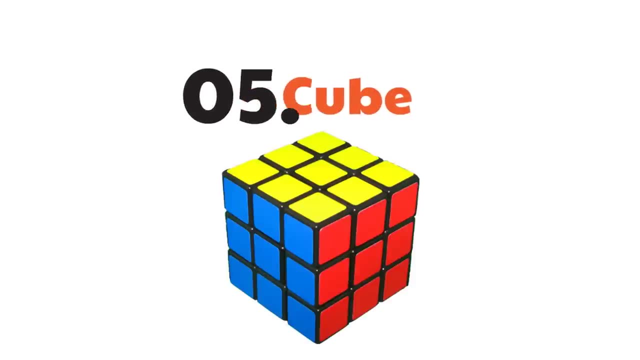 The shape of a cube, Six sides or faces, All squares. I mean, there you go, The cube right, The 3D version of a square, And it's got squares all along the sides Right. there are six sides or faces, All squares, And I don't know. 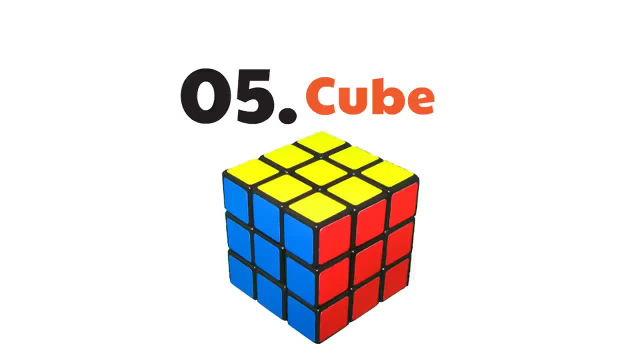 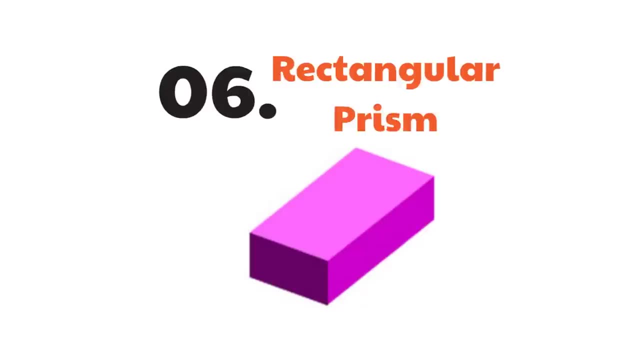 I think it's a pretty cool shape. 2. Music. Our final 3D shape is the rectangular prism. The rectangular prism is the 3D version of the rectangle. It has six sides or faces that are all rectangles. Okay, an awesome example of the rectangular prism are bricks. 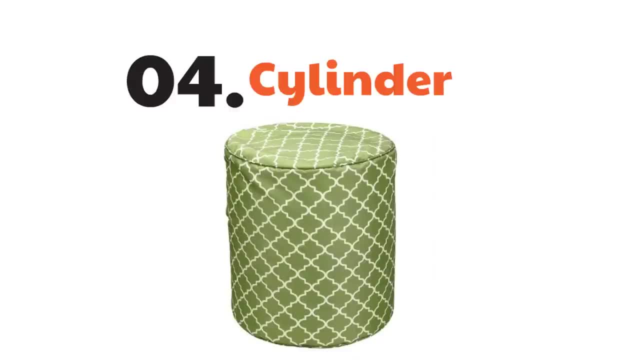 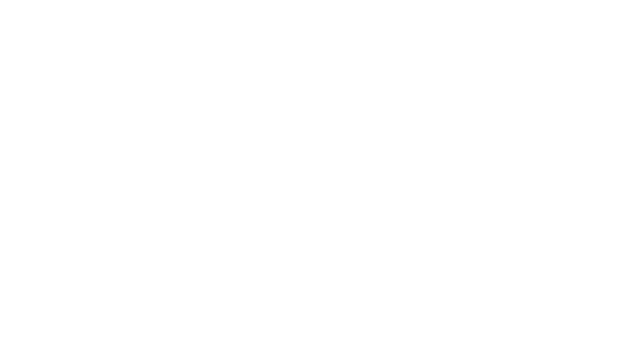 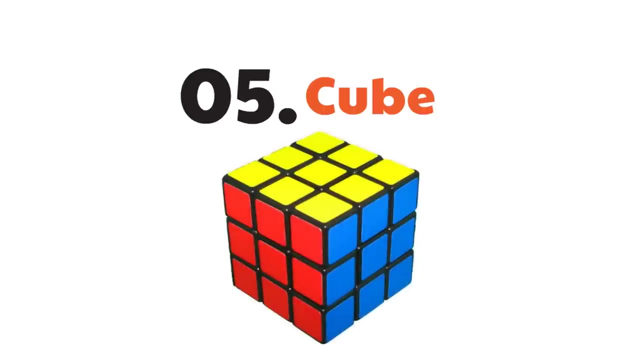 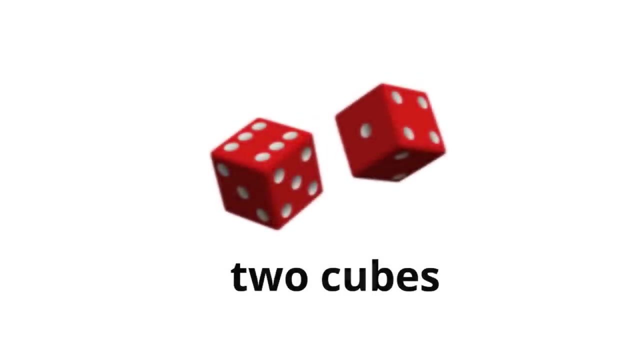 Cylinder. like what in the world do you have to be everywhere? okay, The next 3D shape is the cube. The cube is the 3D version of the square. It has six sides, or faces that are all squares. Here we have two dice. 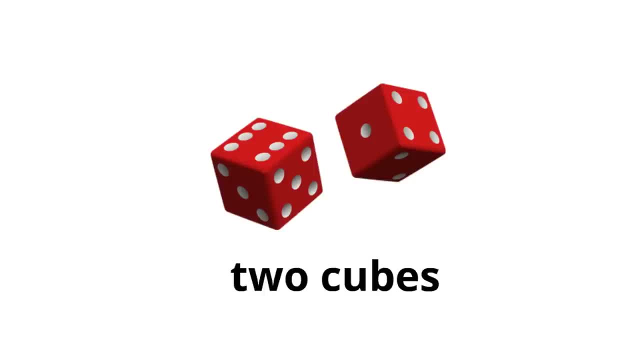 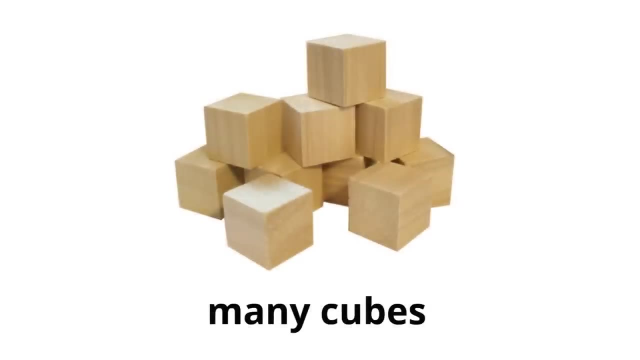 Dice are in the shape of a cube, So these two dice are two cubes. They have six sides, or faces that are all squares. Here we have many cubes. These are cubes that are made out of wood. Each of them have six sides, or faces that are all squares. 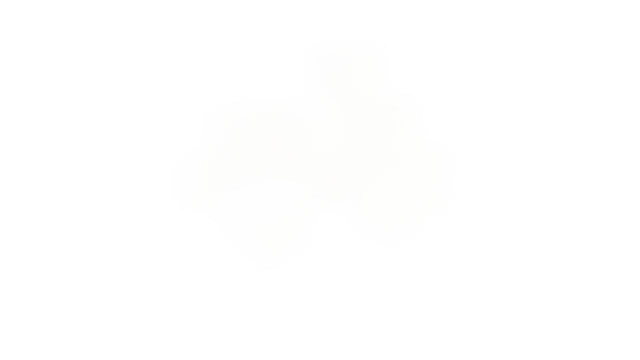 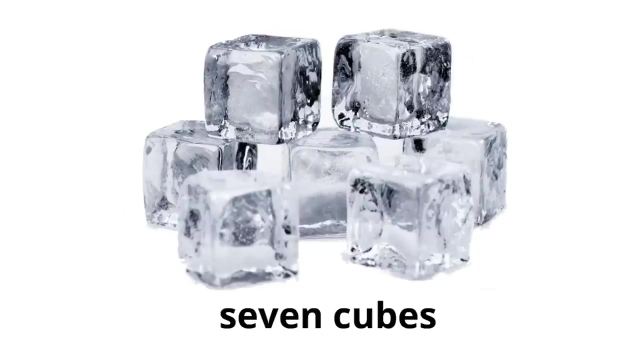 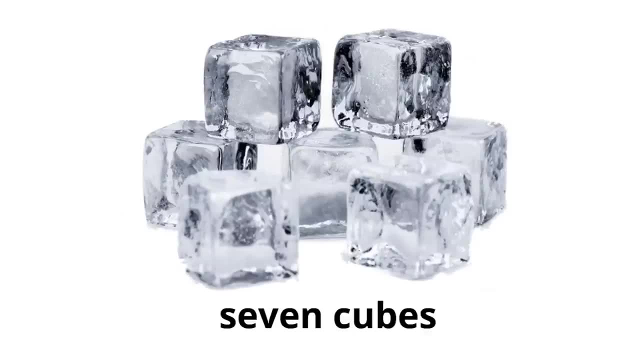 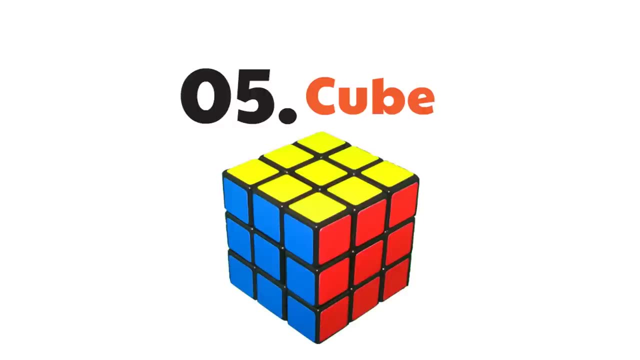 Six sides or faces, all squares. I mean, there you go, the cube right The 3D version of a square and it's got squares all along the sides right. There's six sides or faces, all squares, and I don't know. I think it's a pretty cool shape. 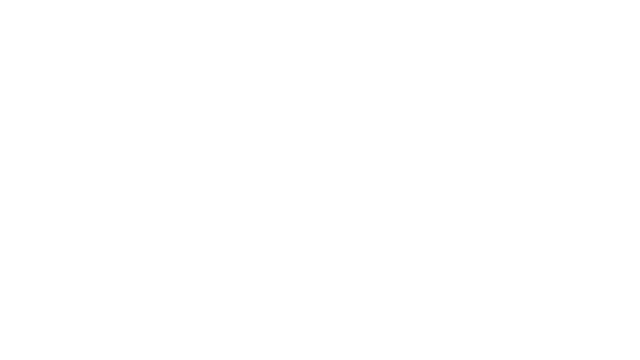 Our final 3D shape is the rectangular prism. The rectangular prism is the 3D version of the rectangle. It has six sides or faces that are all rectangles. Okay, an awesome example of the rectangular prism are bricks, and here we have four bricks. 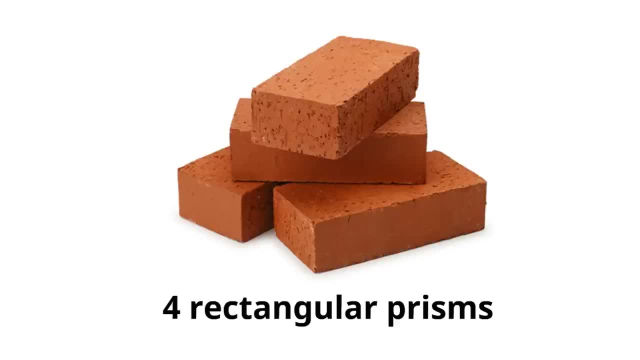 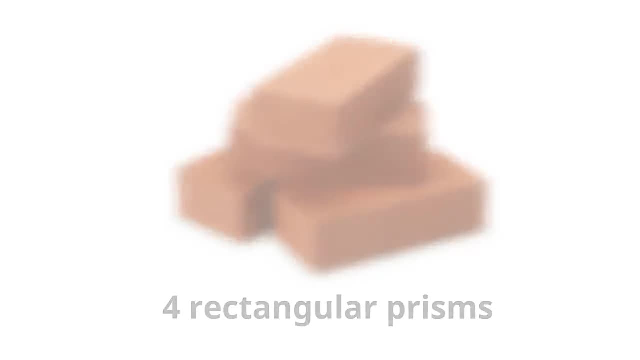 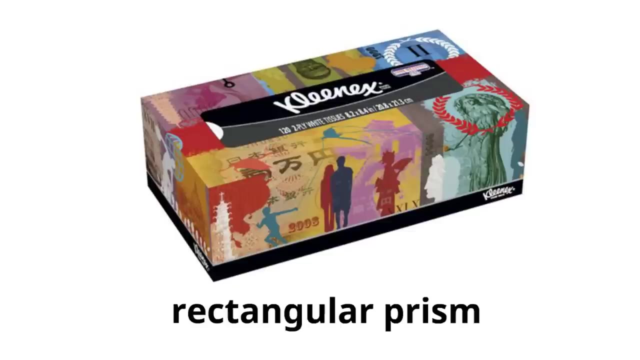 which are four rectangular prisms. The 3D version of the rectangle: Oh, Oh, Oh. You may have seen this in your classroom or in your home. It's a Kleenex box, and the Kleenex box is a great example of the rectangular prism. 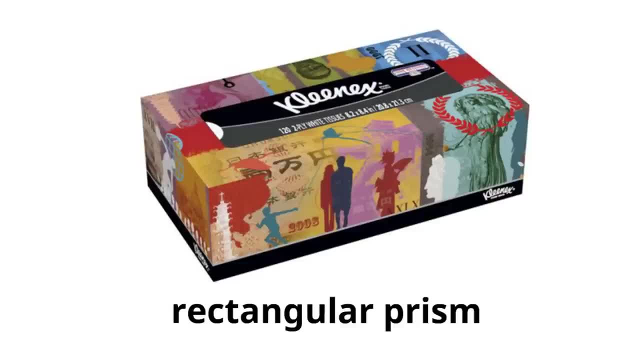 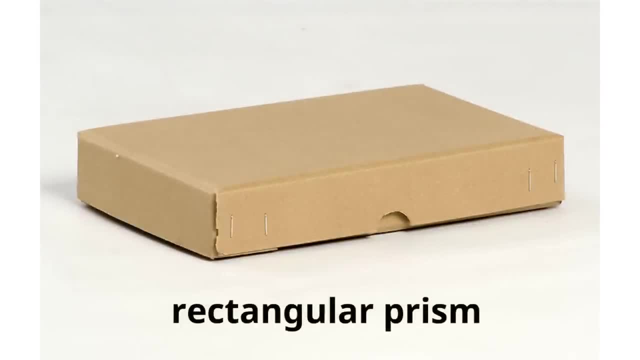 It's got six sides or faces that are all rectangles. Okay, so the secret is, most boxes are rectangular prisms. so here's another rectangular prism and it's a box, and it's a shorter box, but it still has rectangles all around and it's. 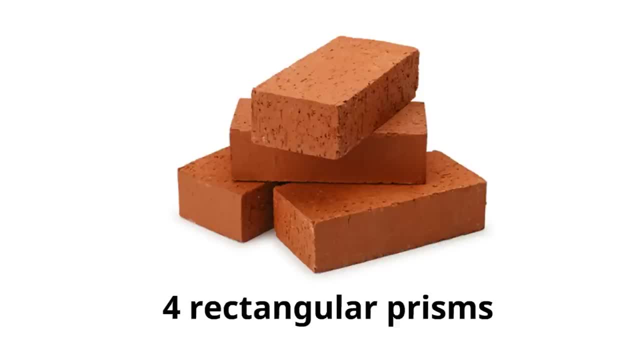 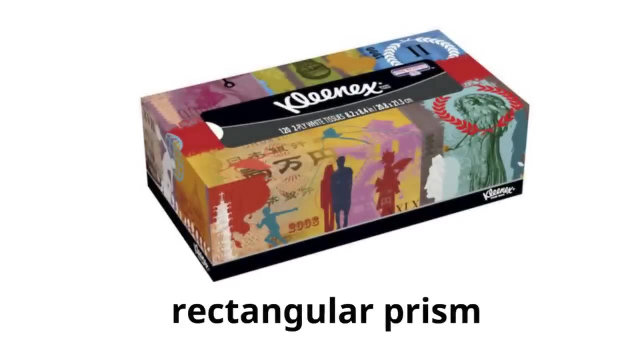 And here we have four bricks which are four rectangular prisms. The 3D version of the rectangle- Oh, you may have seen this in your classroom or in your home. It's a Kleenex box, And the Kleenex box is a great example of the rectangular prism. 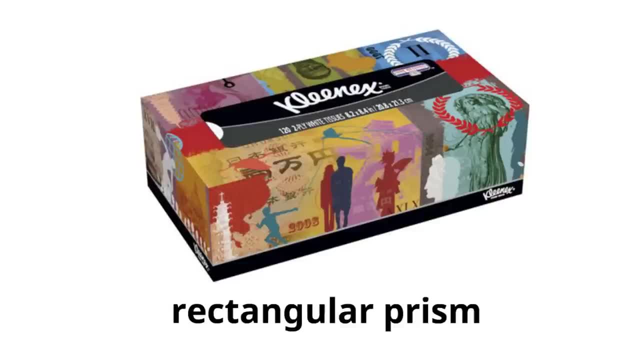 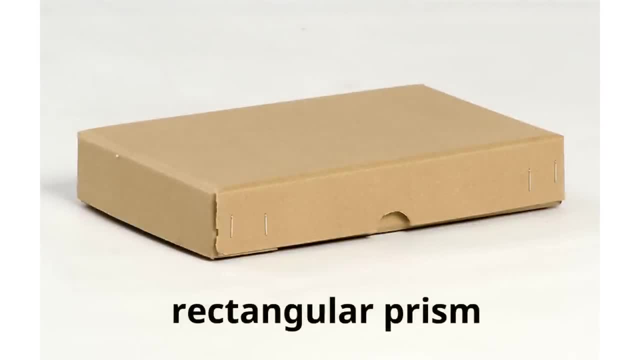 It's got six sides or faces that are all rectangles. Okay, so the secret is, most boxes are rectangular prisms. So here's another rectangular prism And it's a box, and it's a shorter box, but it still has rectangles all around. 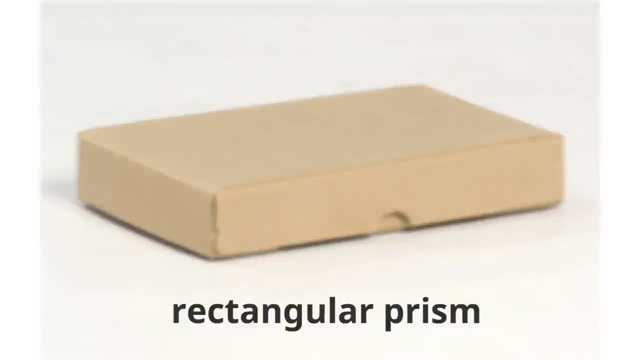 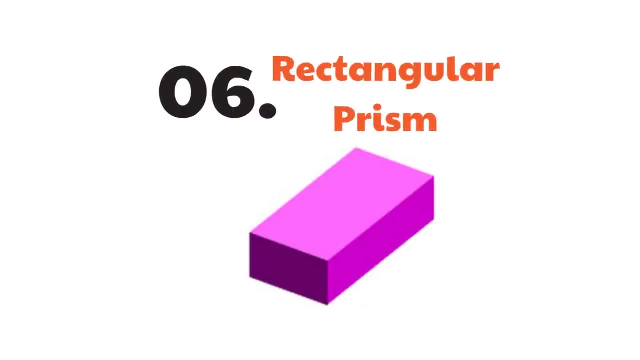 And it's a rectangular prism. What else can we say? It's a cool shape. The rectangular prism is the 3D version of the rectangle. It has six sides or faces that are all rectangles, And it's just a neat shape to have around, I think. 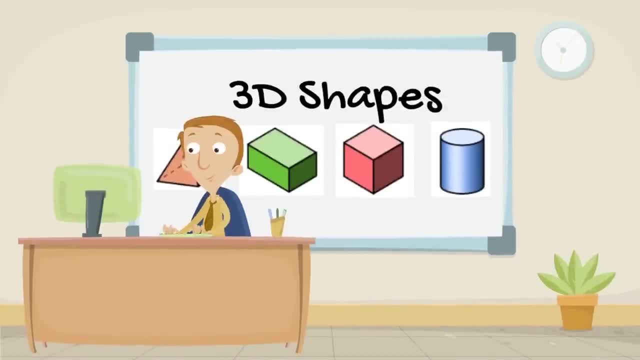 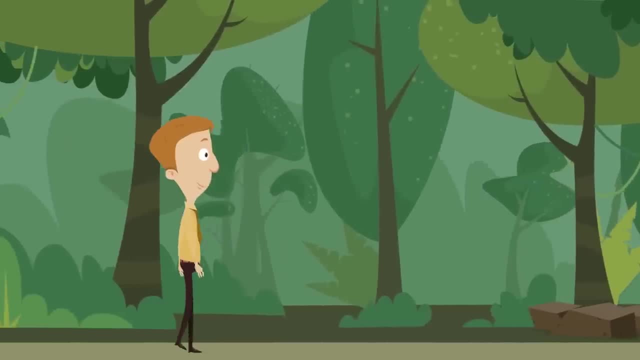 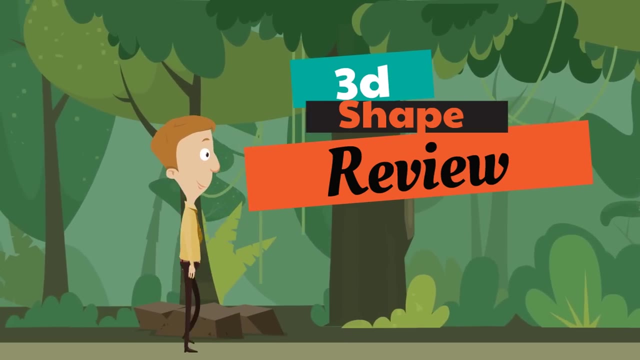 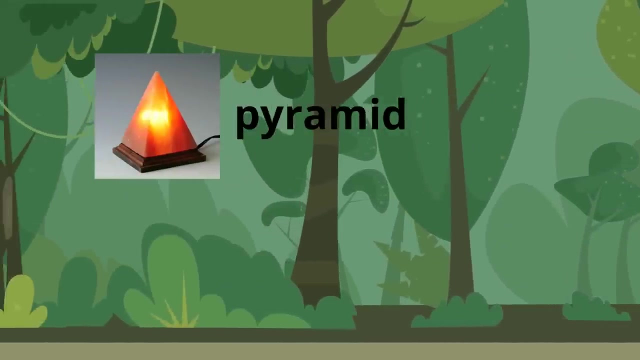 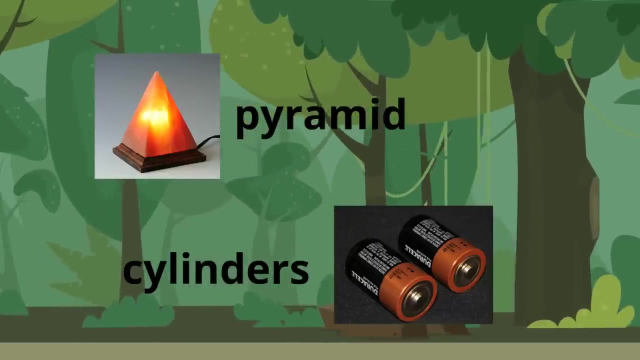 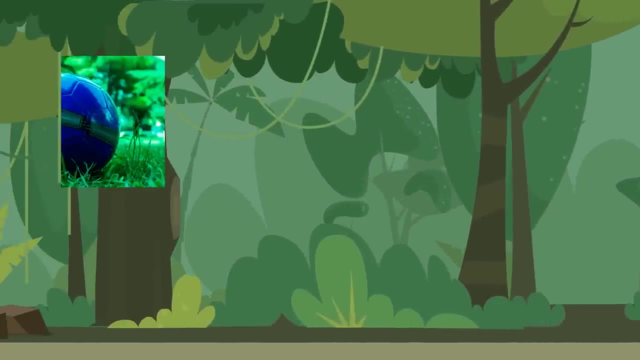 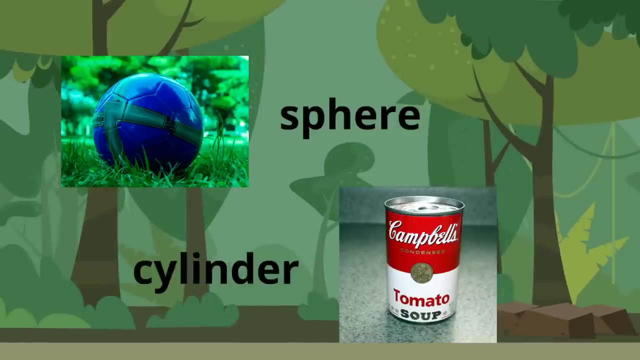 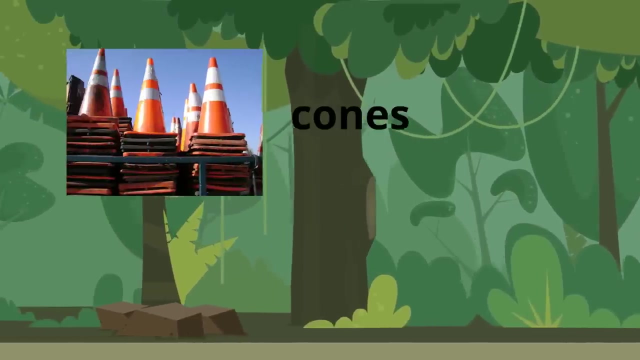 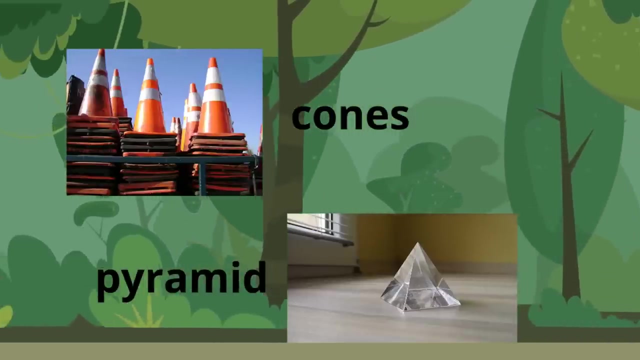 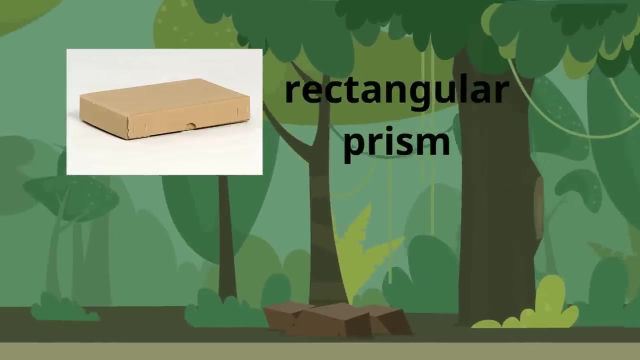 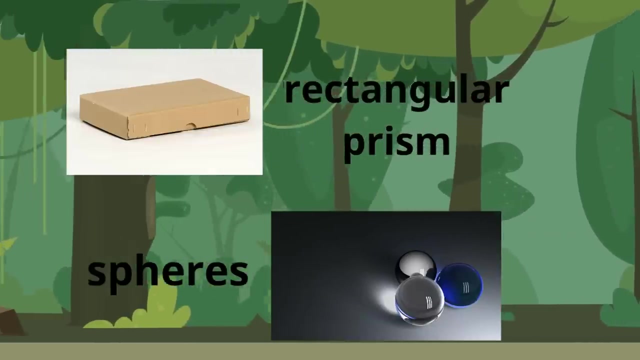 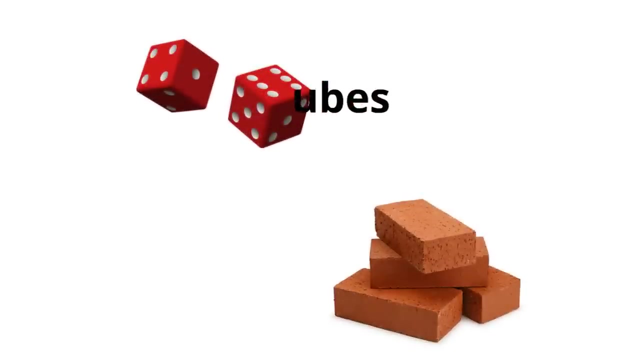 I mean, you know it's cool. So let's review Pyramid Cylinders, Cylinders, Sphere Cylinder, Sphere, Cones, Pyramid Rectangular prism, Spheres, Spheres. let's do some more on the top. here we have cubes. we can tell that because it's. 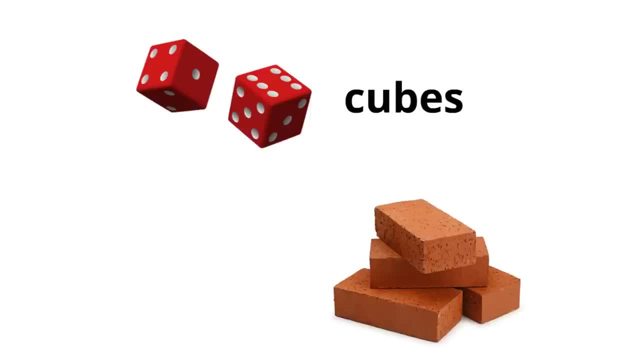 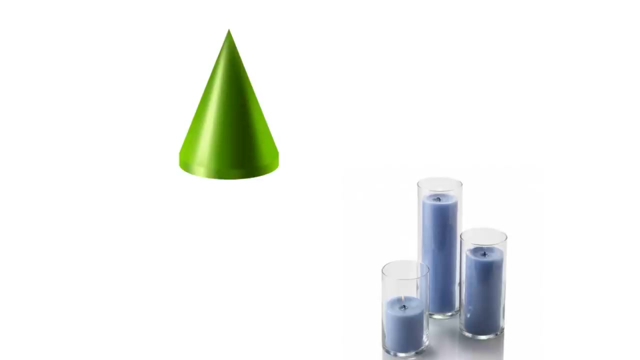 a 3d square. it has six sides or faces. each of them are squares- is pretty cool. do you remember what shape these bricks are? yeah, a rectangular prism. they are rectangular prisms. they're the 3d versions of the rectangle. at the top we have a cone. a cone it's got a circle base on the bottom and all. 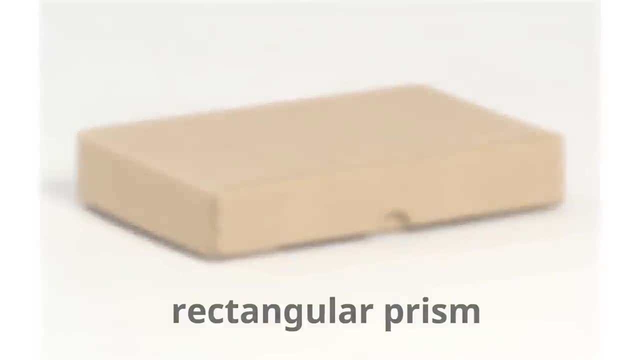 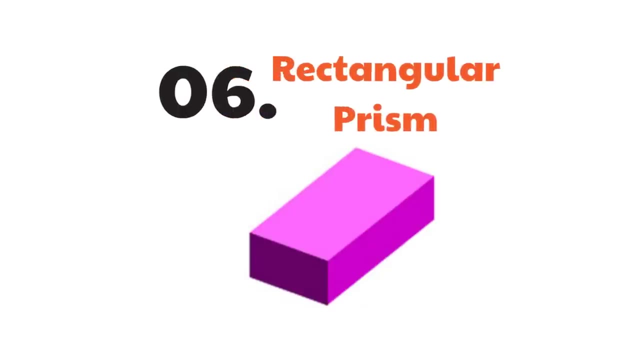 a rectangular prism. What else can we say? It's a cool shape. The rectangular prism is the 3D version of the rectangle. It has six sides or faces that are all rectangles, and it's just a neat shape to have around, I think. 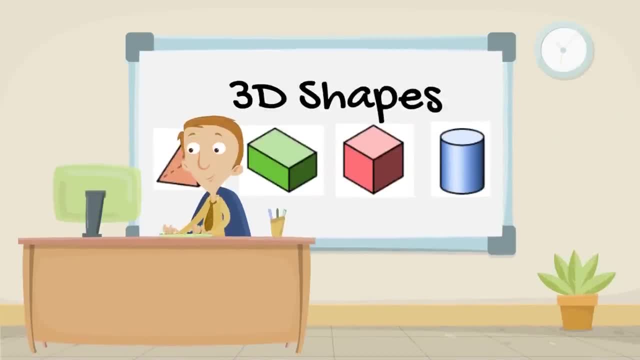 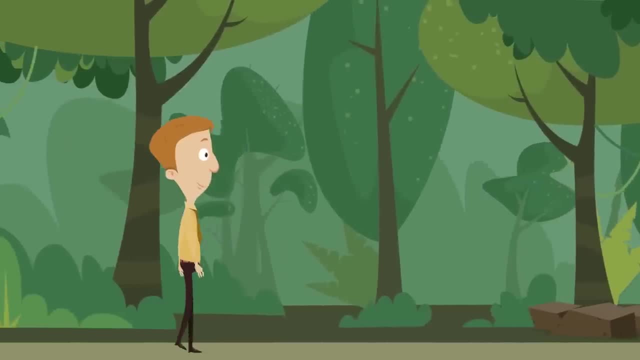 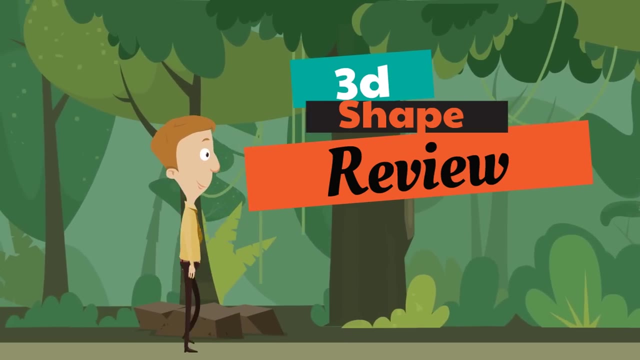 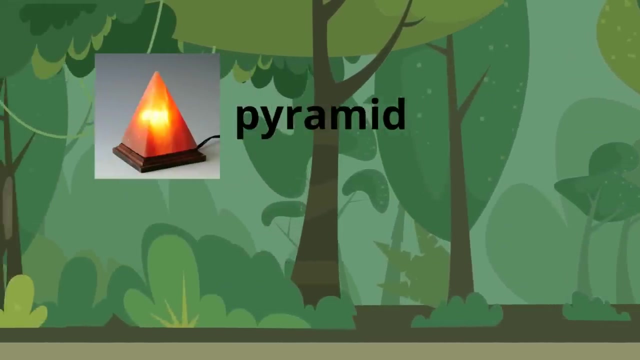 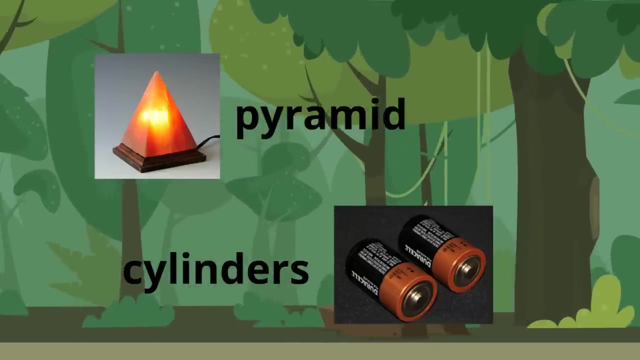 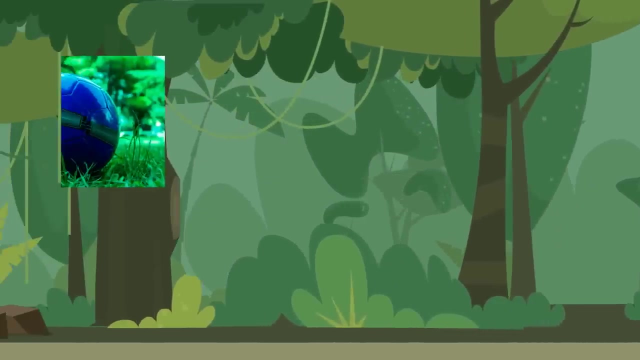 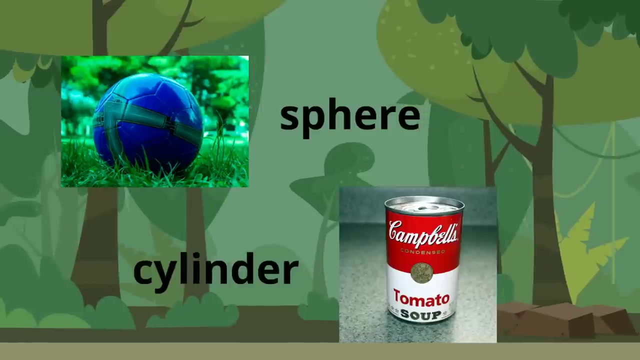 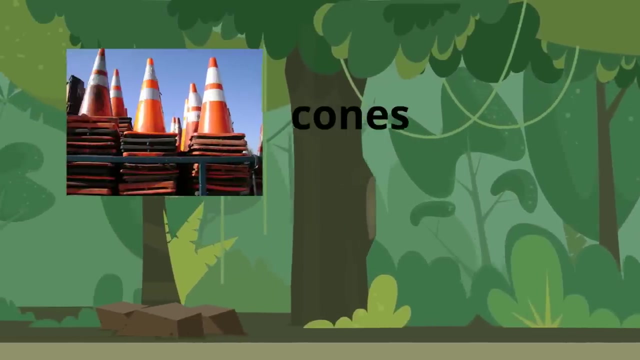 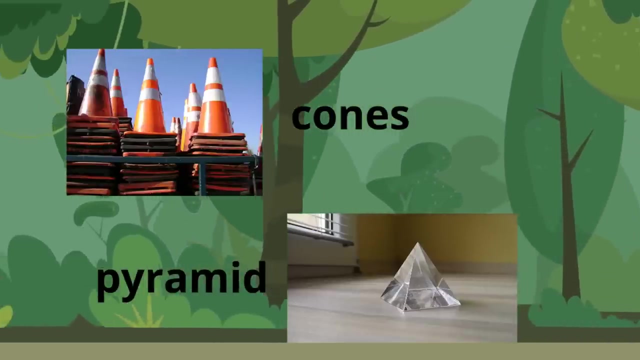 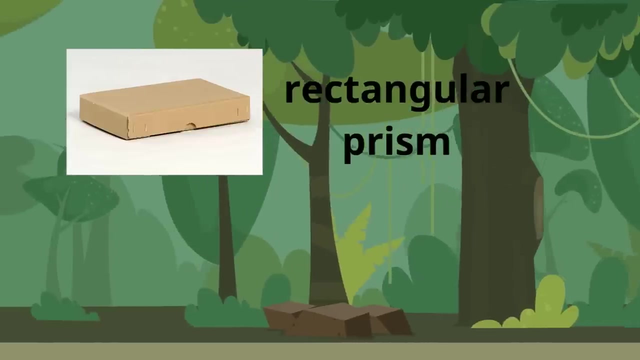 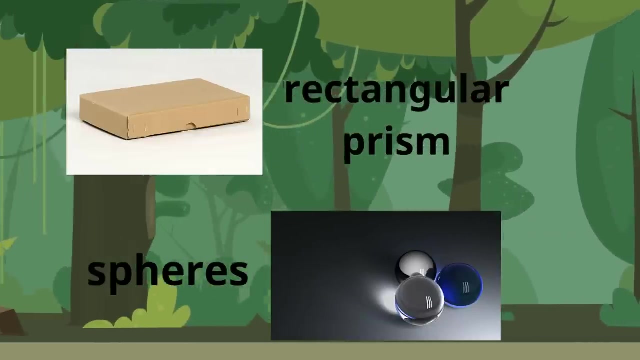 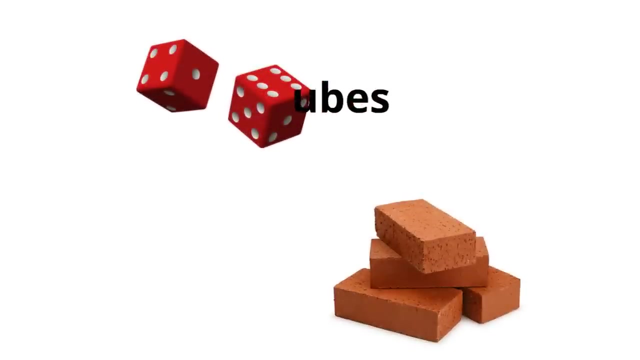 I mean, you know it's cool. So let's review Pyramid Cylinders, Sphere Cylinder Cones, Pyramid Rectangular prism Spheres. Let's do some more On the top. here we have cubes. We can tell that because it's a 3D square. 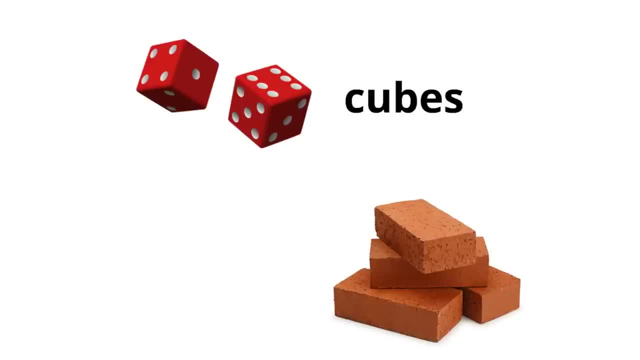 It has six sides or faces. Each of them are squares. It's pretty cool. Do you remember what shape these bricks are? Yeah, a rectangular prism. They are rectangular prisms. They're the 3D versions of the rectangle Rectangular prism. 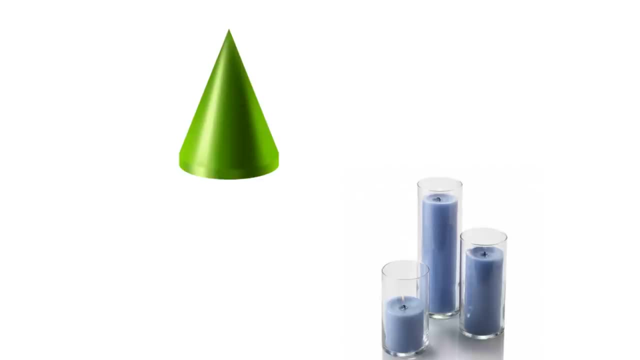 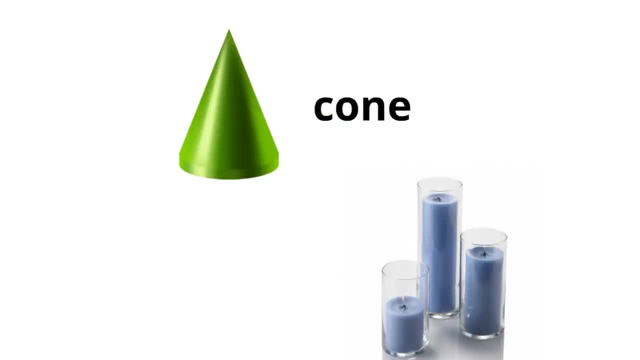 A cone. It's got a circle base on the bottom and all comes up to one point called a vertex. Do you remember the shape here on the bottom? These are three cylinders. They have a circle on the top and a circle on the bottom.